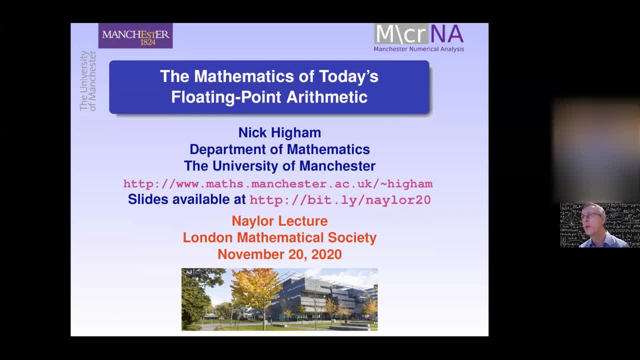 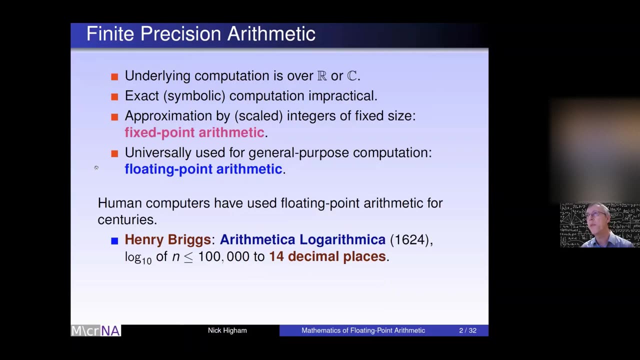 in low-precision floating-point arithmetic that's now quite widely available in hardware And I hope I'll be able to get a little bit of insight into the question of the reliability of low-precision computations. So the context is we have some sort of computation which could be over the 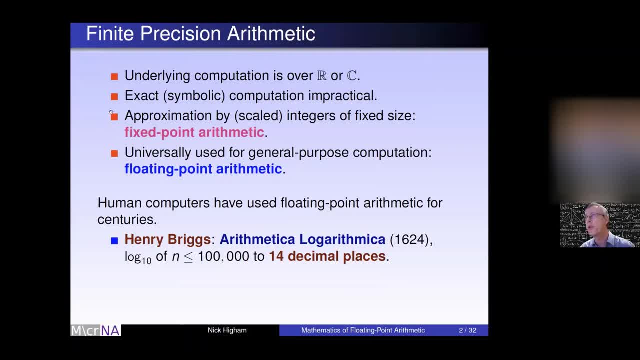 reals or the complex numbers. I'm assuming this is not going to be practical. to do this exactly, which we might typically do in some sort of symbolic arithmetic package, We could work with integers of fixed size with appropriate scale factors. This is still done nowadays. This is known as fixed point arithmetic. 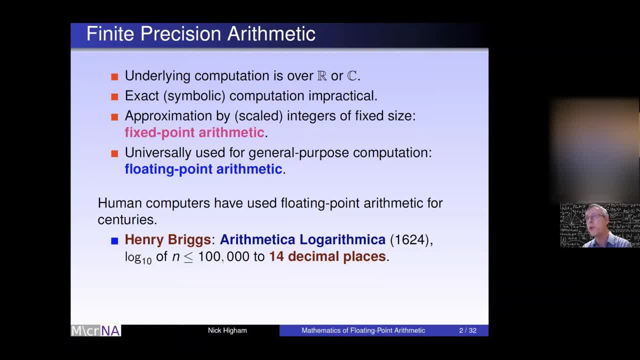 And this is widely used in signal processing in very small-scale devices, But more generally for scientific computing. it's really floating-point arithmetic that we use, And although we've only been doing floating-point on computers for about 70 or 80 years, 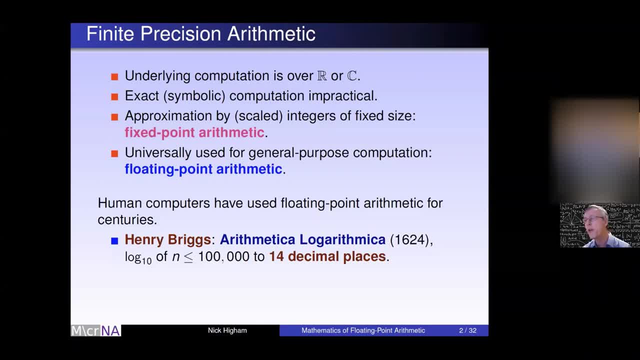 it's just worth remembering that human-centered computing is not just a case of using a single. have been doing this for much longer, and often with quite remarkable results. I mentioned Briggs's table of logarithms, for example, and in fact humans, in some respects, are much better at it than 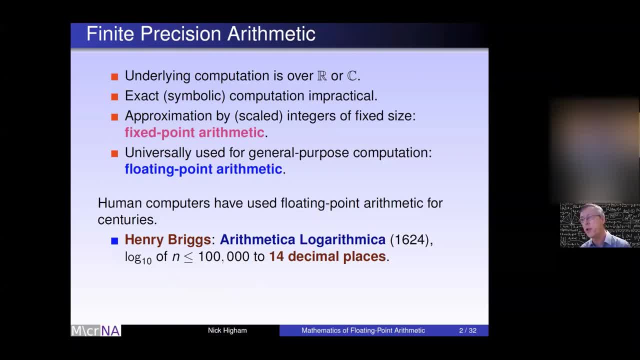 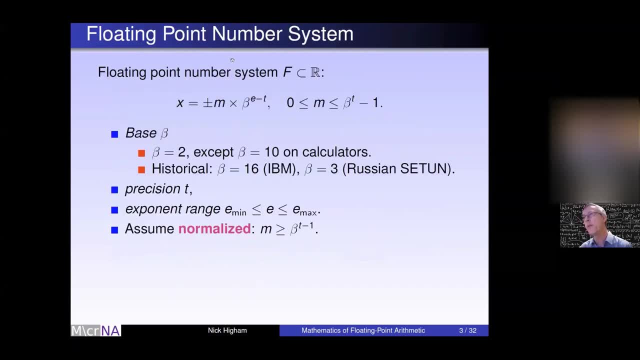 computers in that we're very good at working out how to vary the precision that we need to carry during a calculation. So I'm going to be talking about what I call the floating point number system. So this is a finite subset of the real line, and I like this representation at the top. 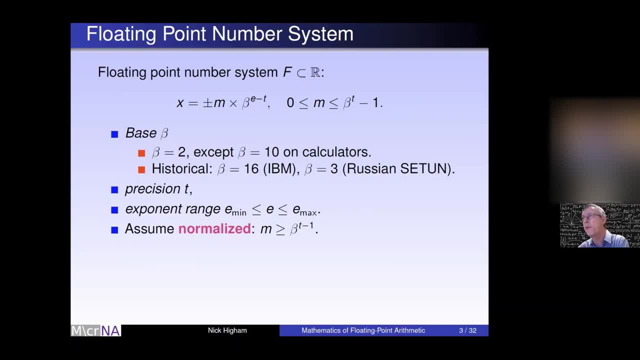 which represents these numbers in terms of four integers. So we have the base beta, which, throughout my talk, will be two, and nowadays is almost always two on all pretty much all machines you're likely to come across. Pocket calculators still use base 10, though, and the reason for that. 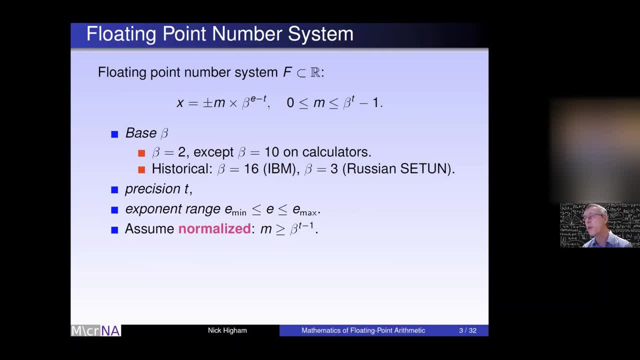 is that they want to avoid conversion errors. So if calculators used base two internally, because we type in our numbers onto the calculator in base 10, there would be conversion errors in before and after the computation is done, which could lead to confusion amongst users who are not. 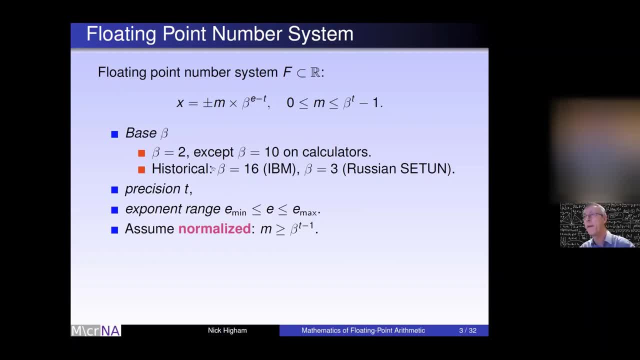 experts in numerical analysis. So calculators use base 10.. Historically in the past, IBM machines often used hexadecimal base 16 and there was even a Russian computer used base 3, but nowadays it's pretty much base 2, which I'll take throughout the talk. We have the precision t. that's another. 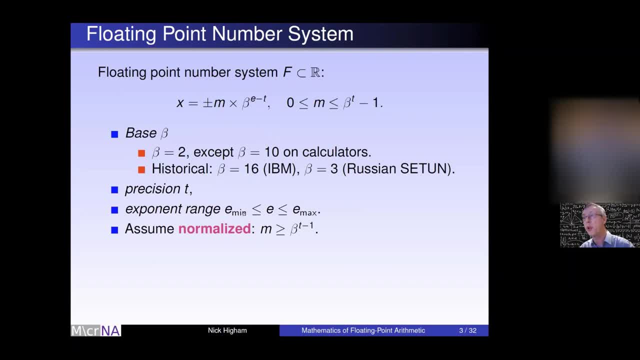 integer. The exponent is an integer lying in this range between e-min and e-max, and I'm going to assume that the numbers are normalized so that m is at least beta to the t minus 1, and this just ensures that we have a unique representation for each number in f. 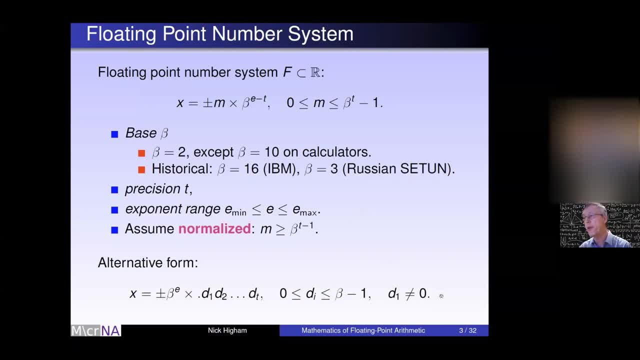 You might see another representation. this is quite common in numerical analysis textbooks. this one at the bottom where we write down the individual digits of our number in base beta. So this, sometimes this is more convenient, but I think generally the the representation at the top is more mathematically elegant and often can leave to 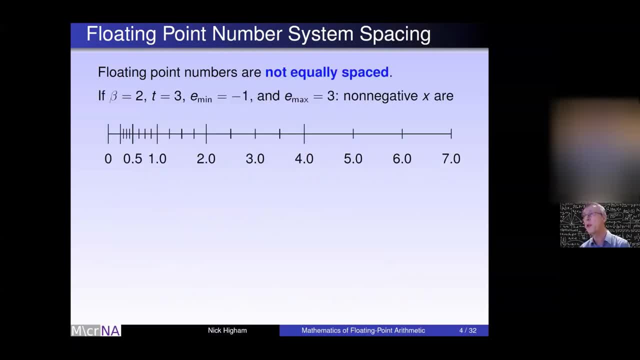 shorter proofs of results. So here's an example of a toy system. I've taken base 2, three digits in the mantissa, or the significant and my exponent ranges between minus 1 and 3, and what I'm showing you with the ticks are the non-negative numbers in this system: f and well, there aren't very many. 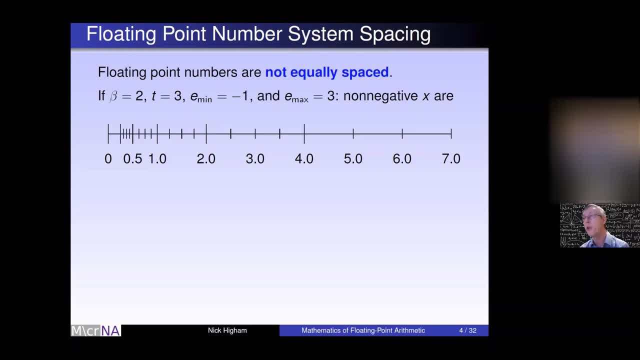 of them is the first thing to notice. but I guess the most important point to realize is these numbers are not equally spaced. In fact, the spacing jumps every time you hit a power of two. So at 0.5, jumps to a quarter, jumps at 1, it jumps at 2, jumps at 4.. So this means that the appropriate measure 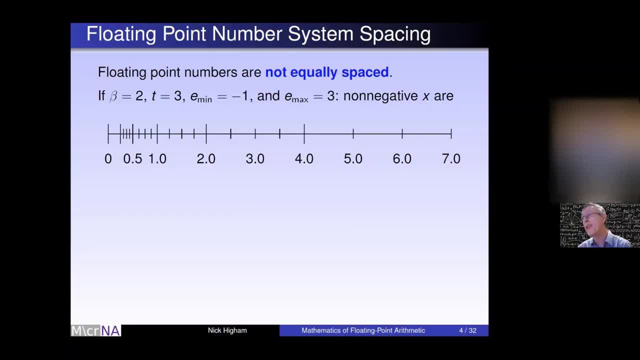 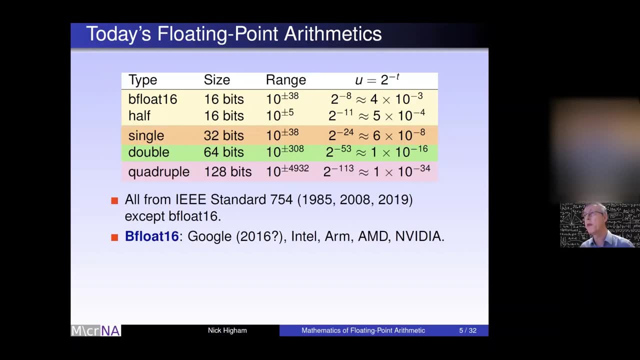 of error when we're working in the floating point system is definitely a relative error, because relative precision is relatively constant throughout the range. So here's a summary of what's available today. For many, many years we've had single and double precision on our computers, and nowadays single means 32 bits, double means 64 bits, and these were 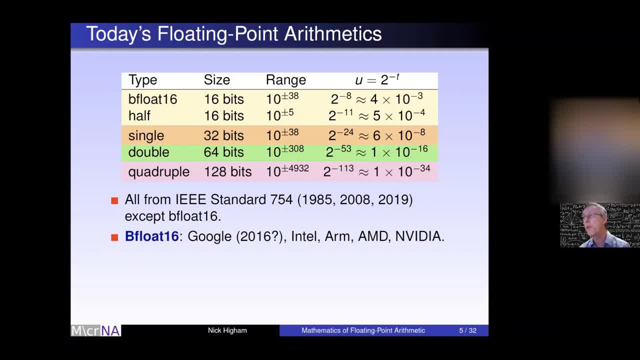 analyzed by an IEEE standard in 1985, and that standard has been renewed a couple of times, most recently last year. The 2008 standard introduced quadruple 128-bit words, but this is mainly only available in software nowadays, so it's rather slow, but everything else I've shown you here is: 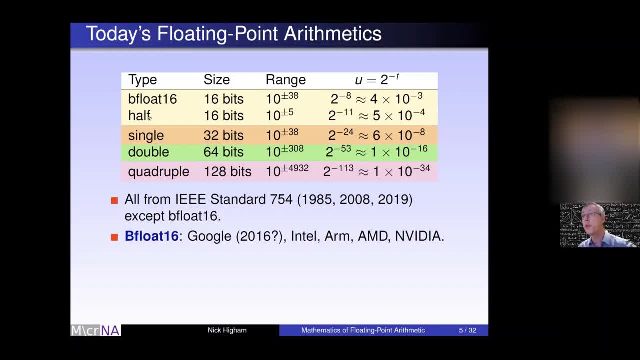 available in hardware. So half precision was introduced as an IEEE format in 2008 and this is a 16-bit format, and Google introduced a different 16-bit format about four or five years ago, and the main difference between half and b float is the the way they. 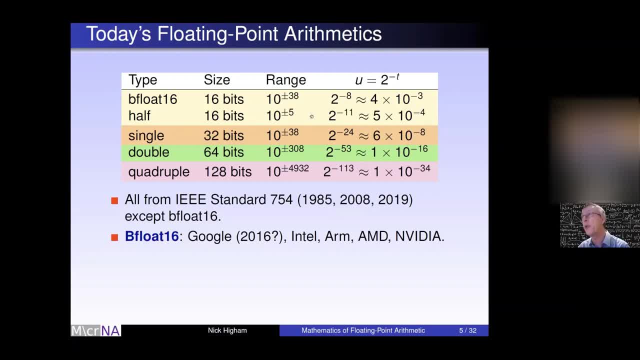 apportion those 16 bits between the mantissa and the exponent. So the IEEE half has a very small range, only down to 10 to the minus 5 and up to 10 to the plus 5, but it has about roughly four decimal digits worth of accuracy or precision. So b float trades some of the precision for range. 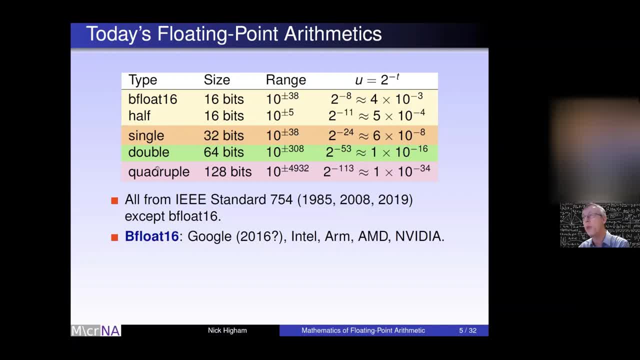 and it has a similar range to single precision. So double precision we can think of that as about 15 digits worth of precision in base 10, half about four. And this b float now is quite widely available on a number of different architectures. Most recently, the NVIDIA A100 GPU now supports it. 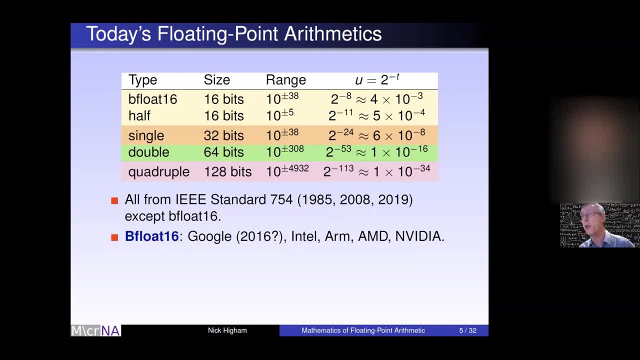 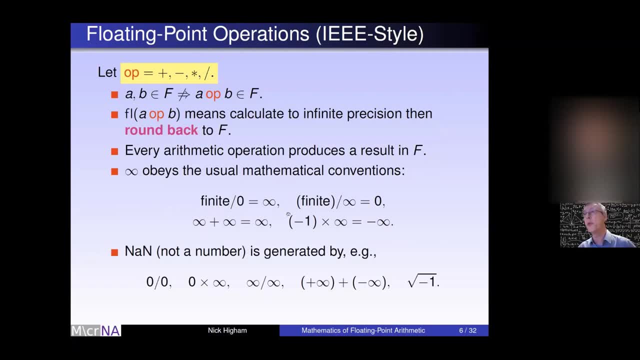 for example. So these things are starting to become widely available, these, these half precision formats. So what are we going to do with our floating bank numbers? Well, we're going to operate with them, and the sorts of operations that we have at the low level are addition. 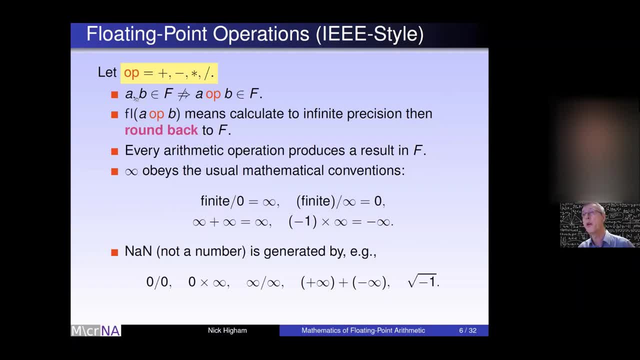 multiplication, division and I guess also square root. But if we do an operation on two numbers in the system then we're not necessarily going to get a number that lies back in in this set f, So we'll need to round it back. So when I write fl, that means the operation of rounding a number back. 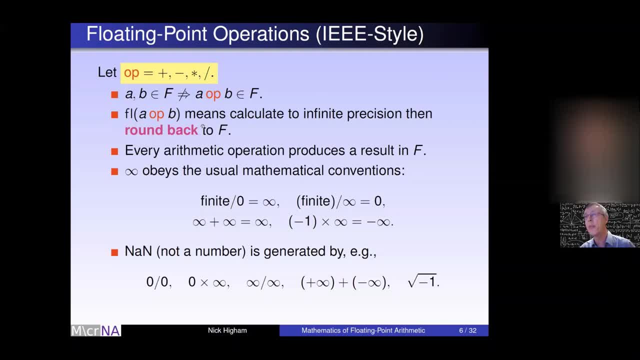 into the, into the set f, And so we can think of this as calculating the answer to infinite precision and then rounding it back according to some rounding rule- and I'll say more about rounding rules in just a moment. So I'm going to assume that we're working in the trepally proposed way. 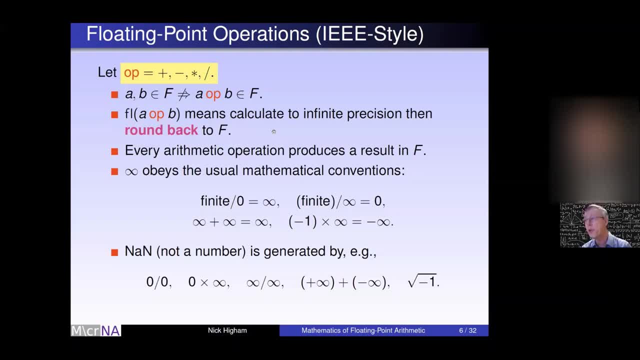 and this means that every operation we can possibly do returns a result in our, you know, set on the item really standard introduces a couple of special numbers in order to achieve this. So we actually have an infinity in entropy and it satisfies these relations here, amongst others. So if you divide 1 by 0, 9 Weekly, you will get this. 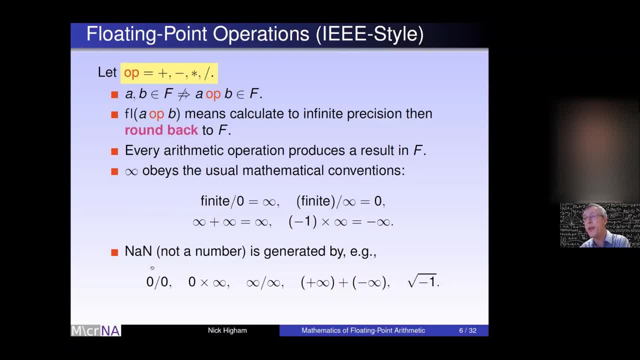 infinity symbol. There's also a number called and none. this is generated by what you might think of as a legal operations like zero over zero. So mathematically this might seem a little bit odd, But the committee that defined the IEEE standard spent many years working on the standard and looking 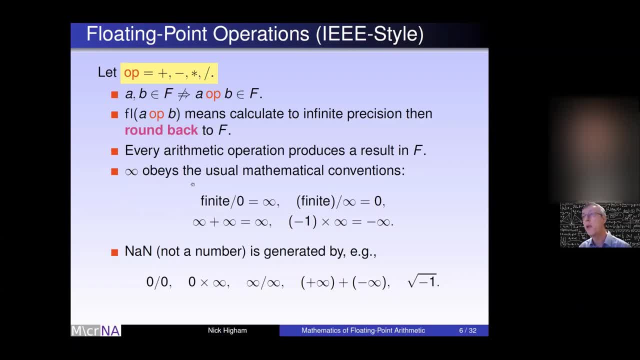 very carefully into the details And this does actually work well. So just to give one example, if you want to program the evaluation of a continued fraction, you normally have to worry about division by zero within the evaluation If you use this rule here that finite over zero is. 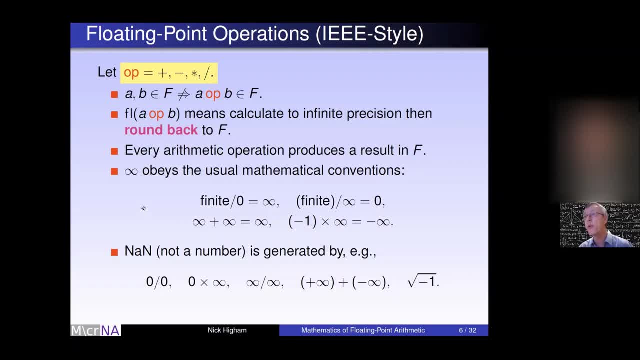 infinity and then one over infinity is zero, you'll find that you don't have to program specially to handle the case of division by zero. you will get the right result when you evaluate your continued fraction. So that's one example of where these these rules are really quite elegant. 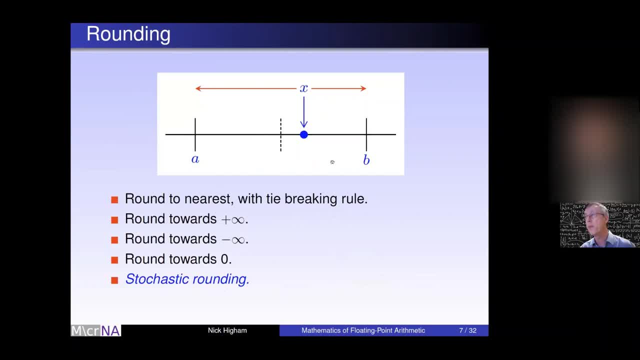 So what about rounding then? So I'm representing in this diagram two adjacent floating point numbers. So A and B are adjacent numbers in F and we have an arbitrary real number, x. we want to round x into the floating point number system. So we want to go. 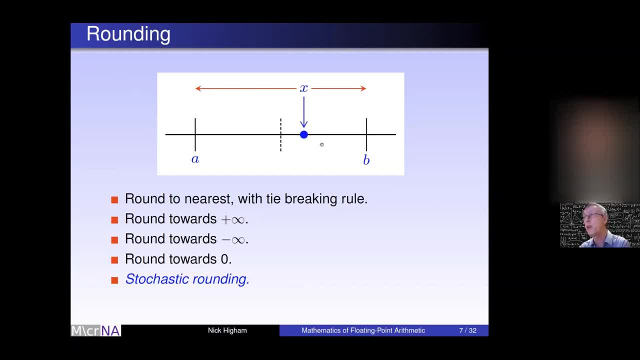 from x to either one of these two numbers, A and B, And I guess the most natural thing to do in this case would be to go to B because it's closer than A. So round to nearest is precisely that you go to the nearest number in F. If you're bang in the middle, then you'll need a tie-breaking rule. 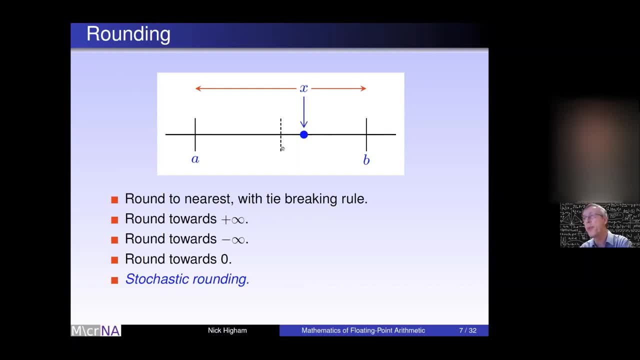 And the normal rule is to round to the number with a zero last bit. That's called round to even. Alternative rules built into the IEEE standard are to round to plus infinity. So in this case we'd round to B, To round towards minus infinity. that would mean round to infinity. 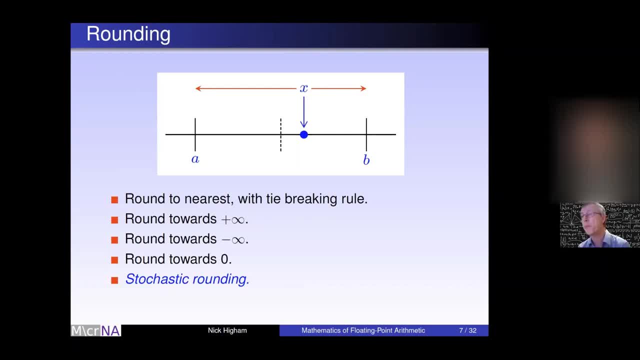 Rounding to A and also rounding towards zero And the round towards plus and minus infinity are very useful for implementing interval. arithmetic. Interval analysis is where you compute an interval in which the true quantity is guaranteed to lie, And so when you do that in floating point, 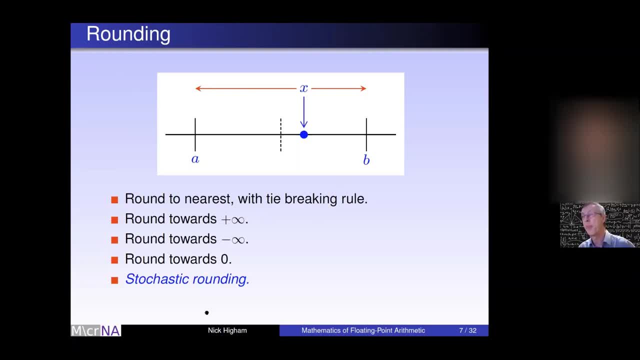 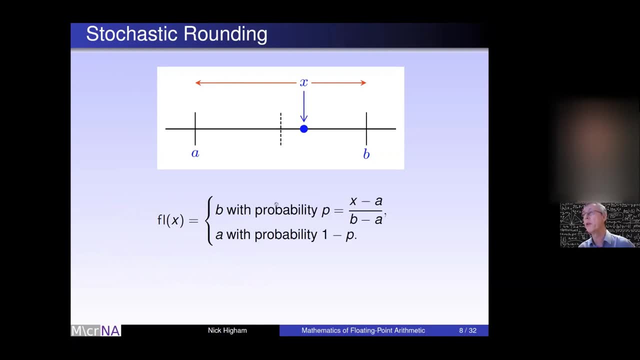 you want to always round the interval outwards. But there's another form of rounding I want to talk about. that's not part of the IEEE standard, and this is called stochastic rounding. And what stochastic rounding does? it doesn't always round to one of A and B. It's a probabilistic rounding, So it rounds. 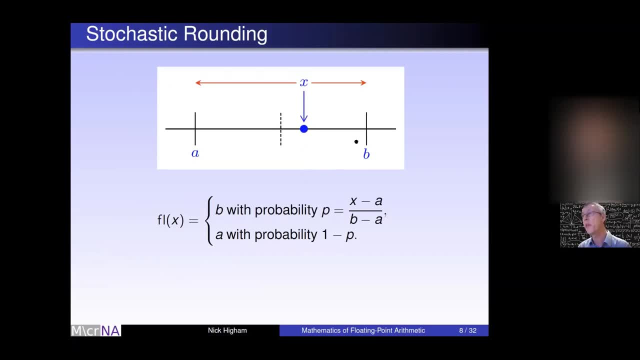 with these probabilities here. So we're essentially saying that because we're closer to B, we're more likely to round to B than A, but we will do so. we will round with a certain probability proportional to the distances to A and B. So this is going to be a different rounding on every call. 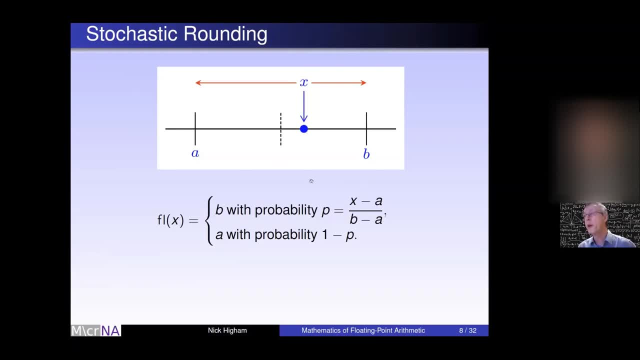 potentially, and it could go to A or B, And at first sight this might seem like an odd thing to do, because in this case if we round to A, then clearly we're making a bigger error than if we round it to B, And so in some sense, locally, that's a bad thing to do. I'll say more about. 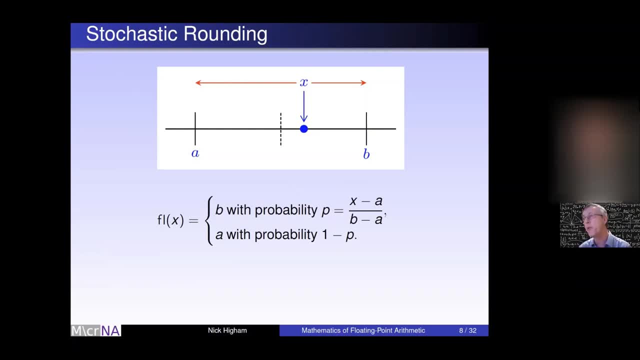 this later. but what will help here is the statistical nature of this rounding and the fact that, on average, we will get a zero error. So I'll come back to that in just a moment. So this is not a new idea. This goes back a long way. 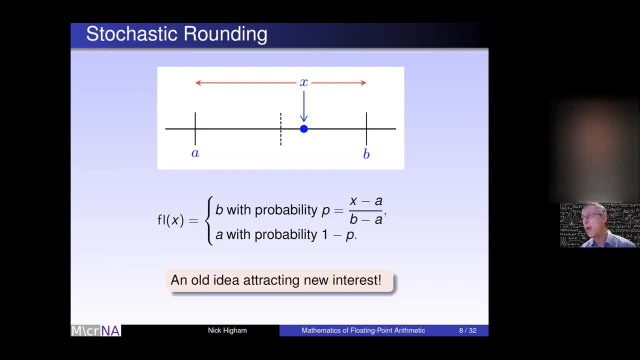 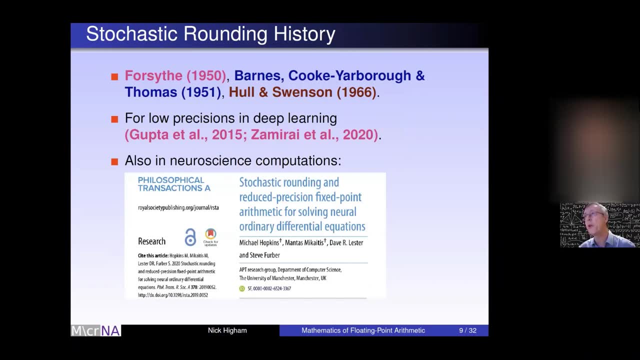 but it's been attracting a lot of interest recently, especially in the area of machine learning. So a brief history. So numerical analysts such as Forsyth, Hull and Swenson were talking about this idea back in the 50s and 60s. Barnes and co-authors were electrical engineers designing 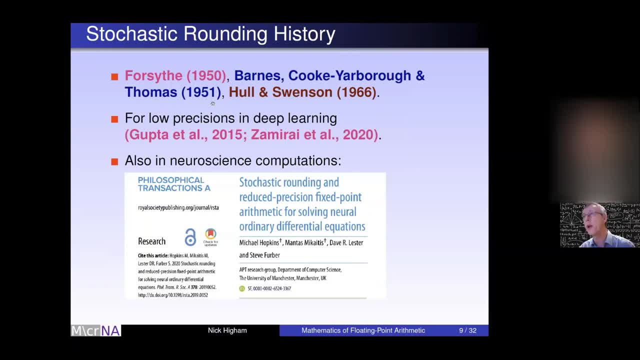 computers, who thought this was actually a good way to round in terms of the implementation. In the last five years or so, people working in deep learning have started to use stochastic rounding in conjunction with low precision arithmetic, finding that it works extremely well, And another 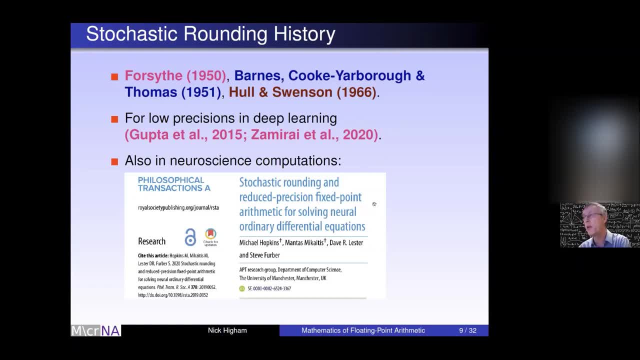 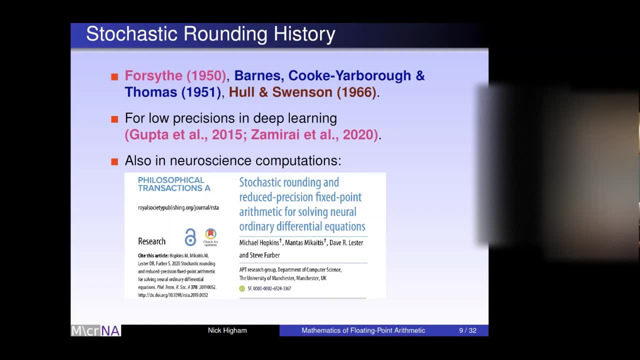 application I want to mention here is from colleagues at Manchester who are working on simulating spiking neurons in neuroscience computations And they're solving differential equations that model those spiking neurons And they don't need low precision. And again they find that stochastic rounding is a good thing to do and it works better than round to nearest. 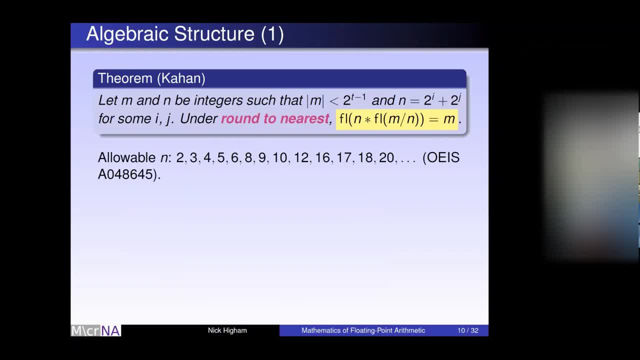 So before I say more about stochastic rounding, I just want to spend a moment asking the question: what is the algebraic structure of the floating point numbers? So my thinking here is that if this set F that I'm talking about happens to be some, 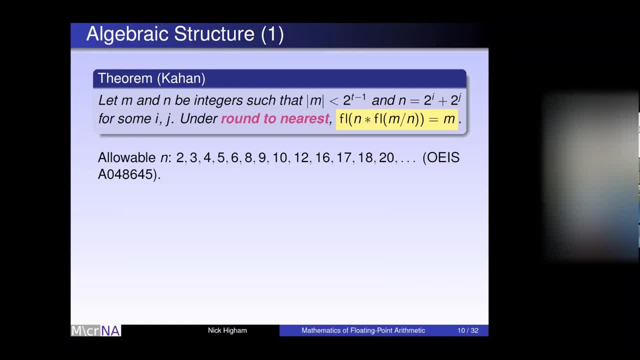 known algebraic structure, then we could take advantage of all the things that are known about it And it might help us in doing our analysis of things like rounding, error, bounds and things like that. So what sort of properties do we have of our system? So I just mentioned 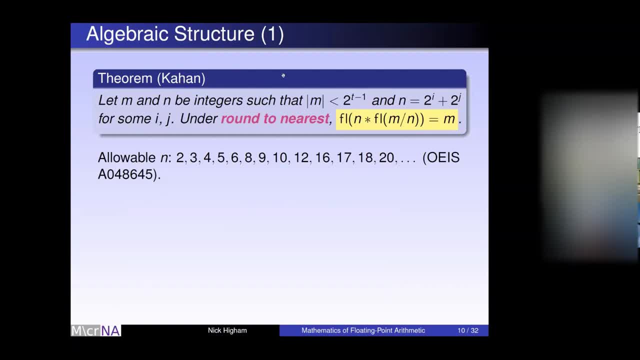 one or two specific examples first of all. So this is a result by Kahan, And it tells you when dividing an integer by another integer, then multiplying by that denominator gets you back to where you started. So if we think of M is one for simplicity. 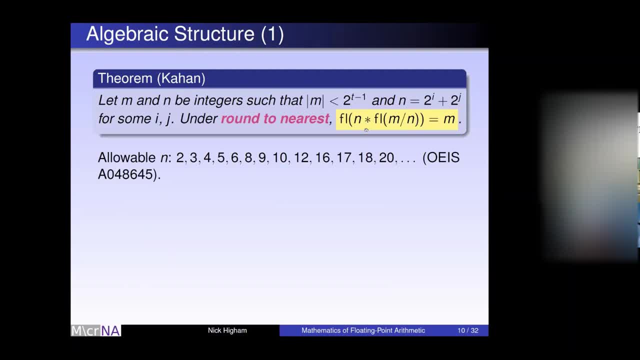 it's when reciprocating, multiplying back gets us back to one, And Kahn's result says that as long as the denominator is a sum of powers of two, then this relation actually holds. So remember, FL means you round back into F each time, And the sequence of allowable N is this: 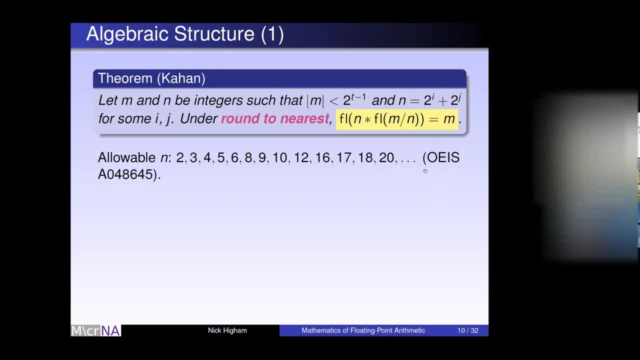 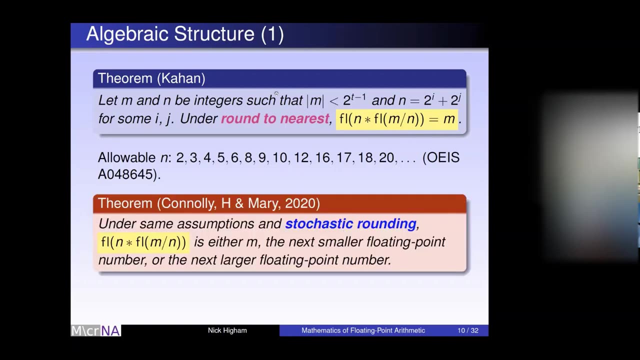 sequence here, And this is actually one of the sequences in the online encyclopedia of integer sequences, not surprisingly So. there's just a certain set of numbers where we can guarantee, with round to nearest, that this nice property holds. You might ask: what about stochastic rounding? This was round to nearest. 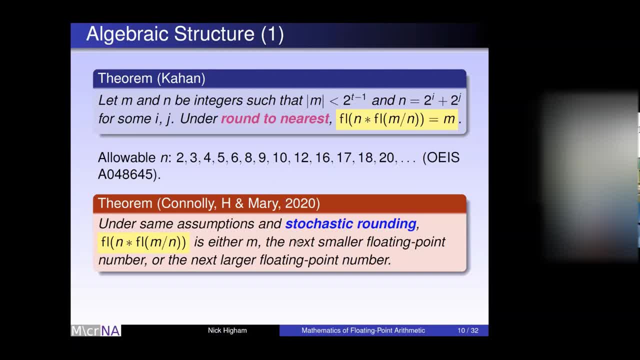 So some recent work with Connolly and Mary under the same assumptions. it turns out that you might get M, but also you might get the next smaller or the next larger floating point number. any of these, These three cases can happen. So things are not quite so nice with stochastic rounding. 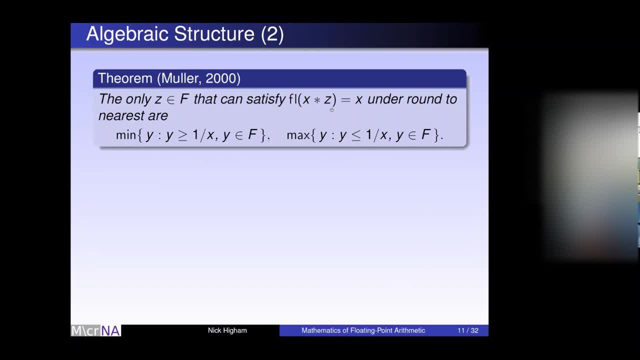 But another view on that same question is a nice result by Muller from 2000.. So if you take a floating point number and you ask what numbers can satisfy x times z is x, so this should be one. then assuming one over x is not a number itself in the system, 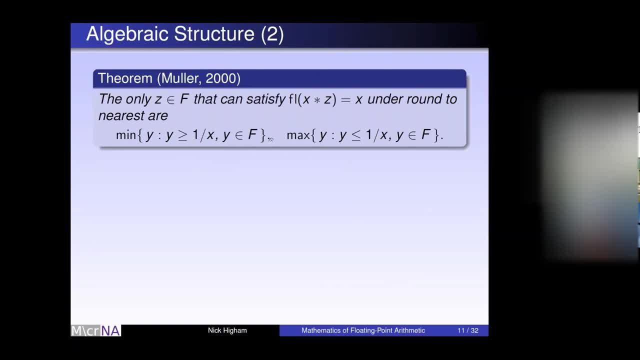 then the answers are the next smaller or the next larger number. They are the only two possibilities for what you might call floating point reciprocals, And in fact they can both occur. So in this toy system with five bits in the mantissa, 3 over 2 actually has two inverses. 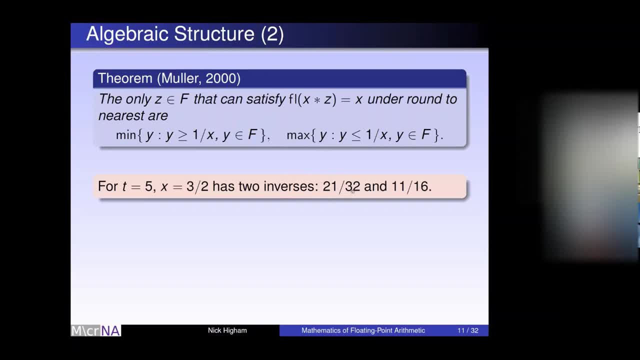 21 over 32 and 11 over 16.. So these are the two numbers adjacent to 2 over 3 in this very small floating point number system. So these are rather weird behaviours. So this is a rather strange set. and I haven't even mentioned yet the fact that addition is not associative. So 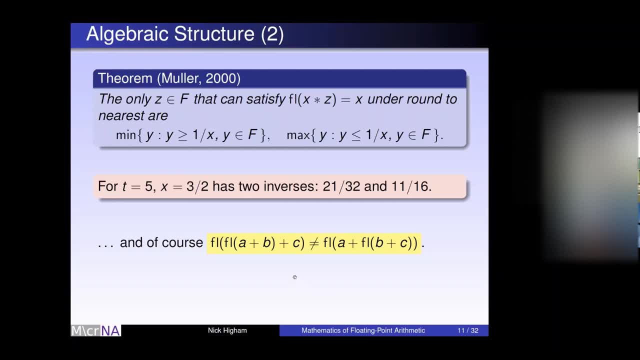 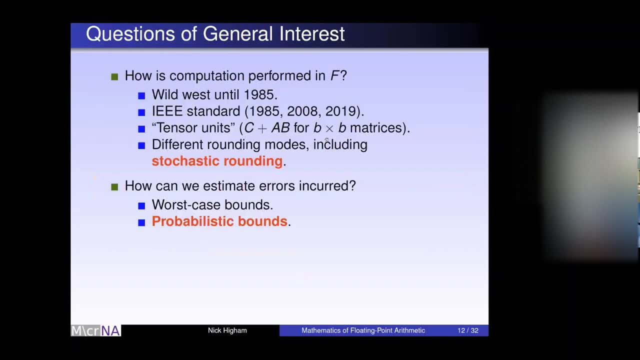 So this is really quite a, in some senses, a nasty set of numbers, and I don't believe it fits into any well-known algebraic framework, unfortunately. So what sort of questions might you want to ask about floating point numbers? Well, there's how you do the computation and then there's how you bound the errors in those computations. 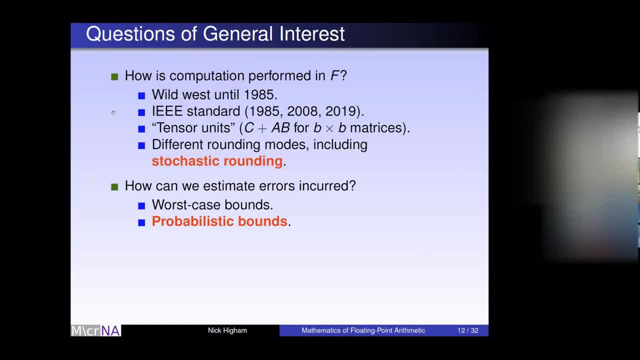 I've mentioned already the IEEE standard. Prior to the standard it really was like the Wild West, with different manufacturers doing different ideas on how to implement even just the basic operations. So the IEEE standard really smoothed things out and for the last 30 years or so we've had a very nice uniform setup on different computers. 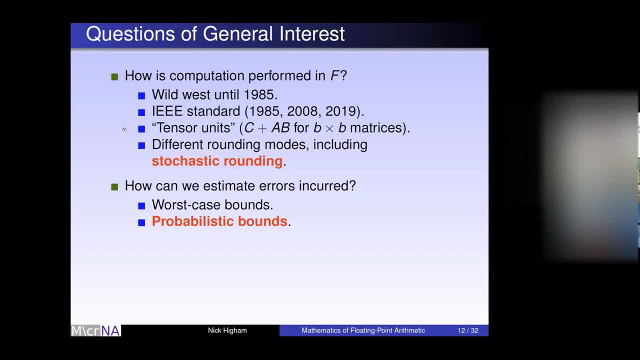 But just recently we've got developments that are making things more complicated again. So Google have their tensor processing unit, NVIDIA have their tensor cores, And what these are is specialist hardware units that can do a little matrix multiply So they can do C plus A times B where C and B are B by B matrices. 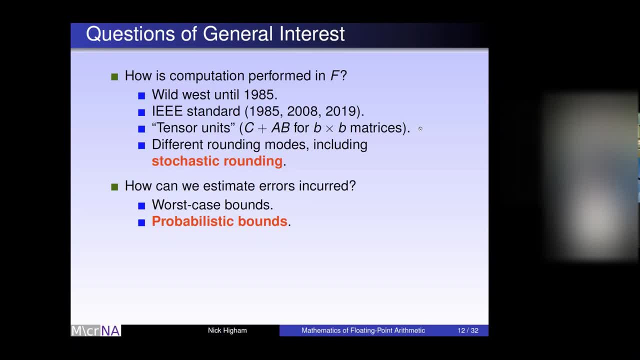 B might be 4 for one of the NVIDIA GPUs, might be 128 for a Google TPU. And they do this very, very fast and in low precision. And to complicate things further, they will accept A and B of, let's say, half precision and return the answer, this sum, in single precision. 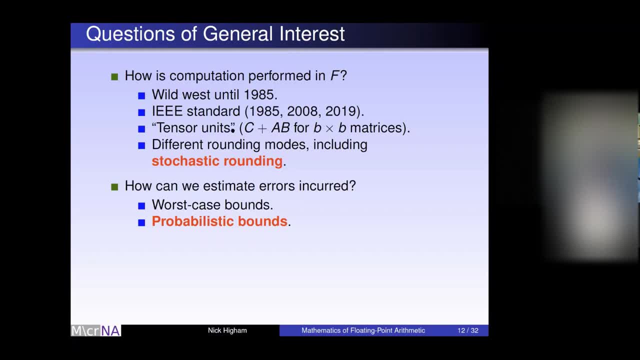 So these are very much multi-precision units That require a much more detailed and more complicated error analysis, And there's also the question of different rounding modes here. What rounding modes are being used within these computations, Stochastic rounding being one of those possible modes? 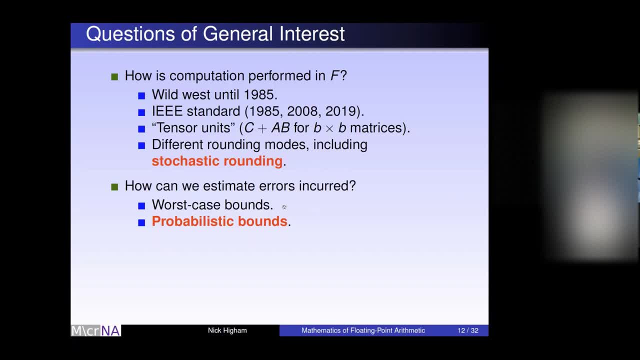 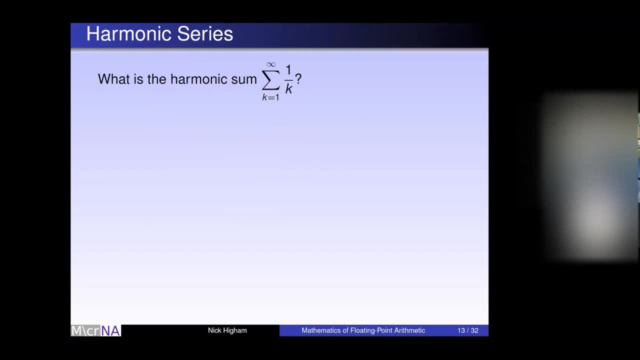 For error analysis. we've got the traditional worst case bounds and also probabilistic bounds, which is what I will talk about in just a moment. But first of all just a quick example that I think is quite interesting. I'm going to compute the harmonic. 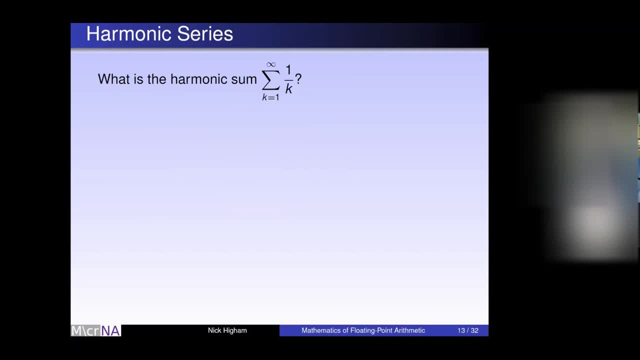 So I'm going to compute the harmonic sum, the sum of the harmonic series. Now, as any first-year undergraduate knows, this sum doesn't exist, The series doesn't converge, the series of partial sums. But it does exist in finite precision because, well, for one thing, there's only finitely many numbers in our system. 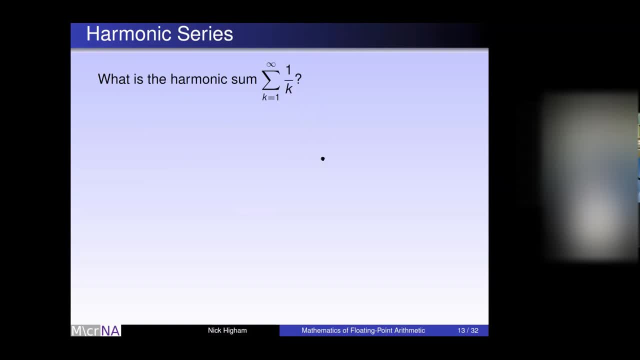 And secondly, once K is large enough- 1 over K- will underflow to zero, So we do expect to get a finite sum. So the fun question is what happens if you compute the sum in different precisions, So if we do it in the lowest precisions of a half? well, with the BFLOAT format, after just 65 terms, this series has converged, meaning that the next term- 1 over 66, will not change the partial sum computed so far. 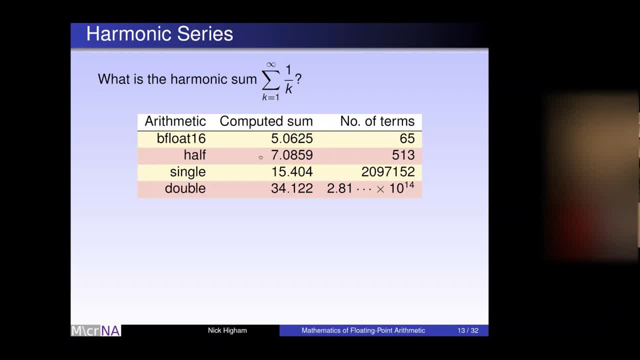 So the sum settles down at this value. With the IEEE half format, which is a bit more accurate, you can go for 513 terms. Simple precision gets to a value of 15.. This can be done in a few minutes on a desktop computer. 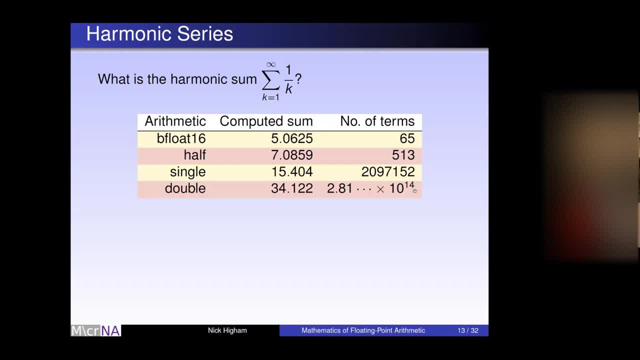 And the double-precision calculation was done by Malone and it took him 24 days on his desktop, because there's an awful lot of double-precision numbers So widely differing results from these different arithmetics. What about the different rounding modes? 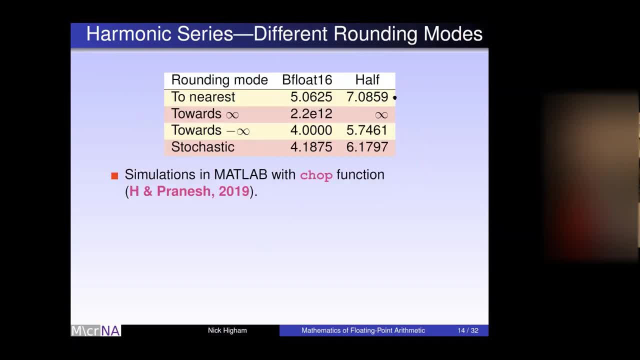 So if I focus on the half-precision formats- now, this is the first line- is the one we just saw with round to nearest. If we round every result to plus infinity, then the half-precision one blows up. BFLOAT 16 is still there. 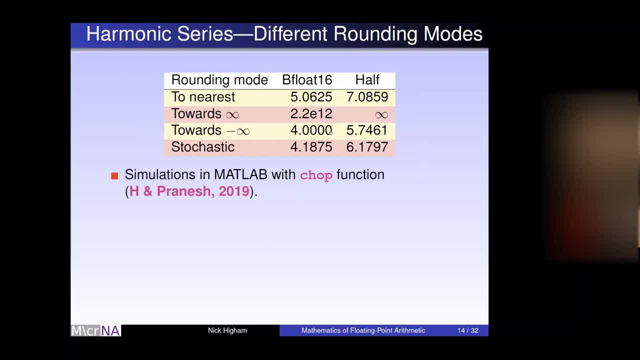 It's labeled, to a computer-finite sum Rounding downwards towards minus infinity. we of course get smaller numbers, but these values here And stochastic rounding. the particular run I did here was somewhat in between these different values And these were all done in MATLAB with a package that Sri Pranish and myself have developed that can do different rounding modes. 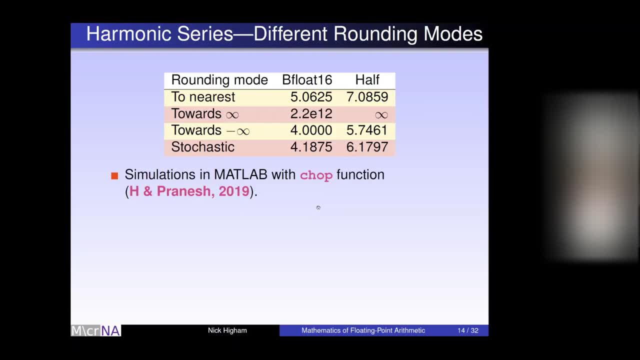 So the message from that example is that we're getting very different results- actually unusually different results- just by changing the rounding mode or changing the arithmetic. But of course it's a little bit hard to interpret what's going on, because the fact is that for each different precision I'm really computing a different sum, a different finite sum. 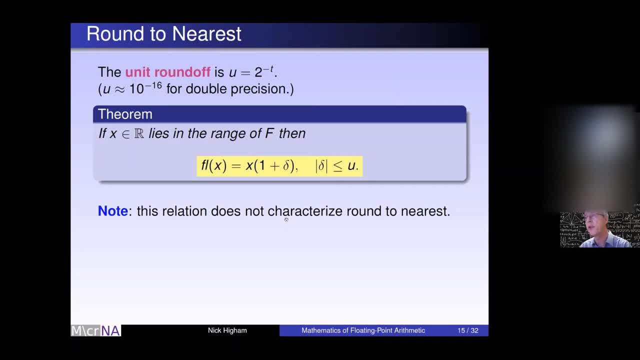 So let's now look in a bit more detail into trying to understand the effects of these errors. So rounding shown here, here's a result that tells me what is the error in rounding. So I take an arbitrary real number. I want to round it into my number system: F. 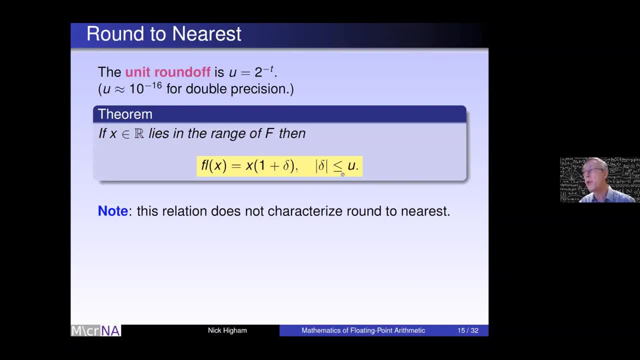 And the result says that the relative error delta is bounded in modulus by the unit round-off And the unit round-off is given by 2 to the minus t. t was the number of bits in the mantissa And this is, for double precision, about 10 to the minus 16.. 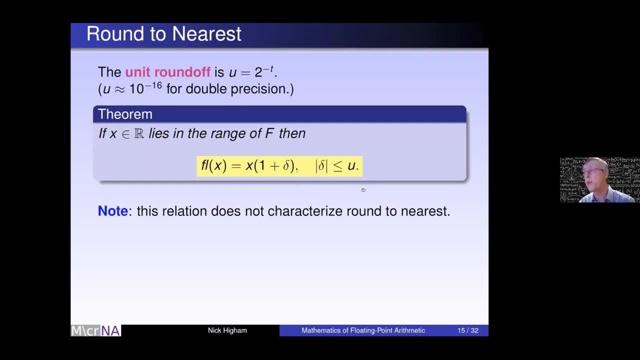 So every rounding has a little relative error of about 10 to the minus 16.. I hasten to add that this result here doesn't actually characterize rounding. It's just something that rounding nearly satisfies. But there are of course many deltas that satisfy this. 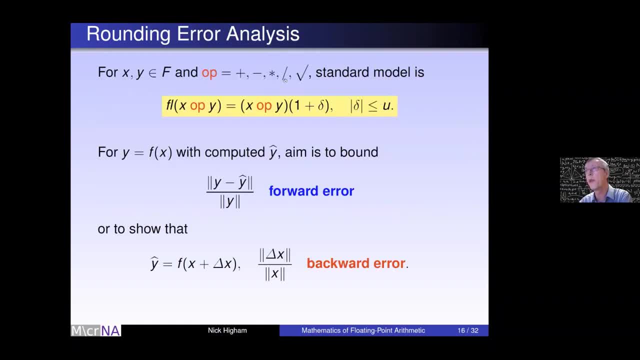 But there are many deltas that satisfy this inequality. What about the round? What about the computation of the elementary operations: Add times, divide and even square root? Well, if we do what the IEEE standard suggests, we compute the answer to infinite precision and then round it back into our system, then of course we get this result here. 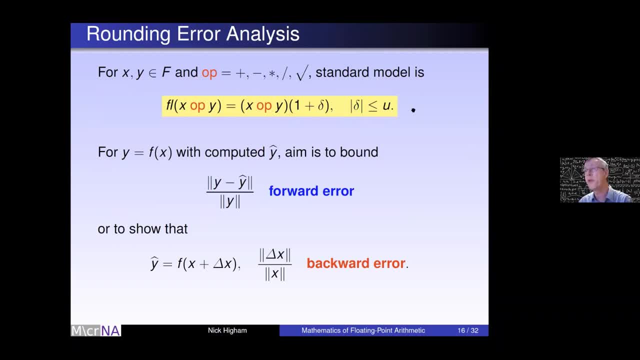 This is just rounding the true x up y And this is satisfied for all modern computer systems, This condition here. So this is just rounding the true x up y And this is satisfied for all modern computer systems. So this is just rounding the true x up y. 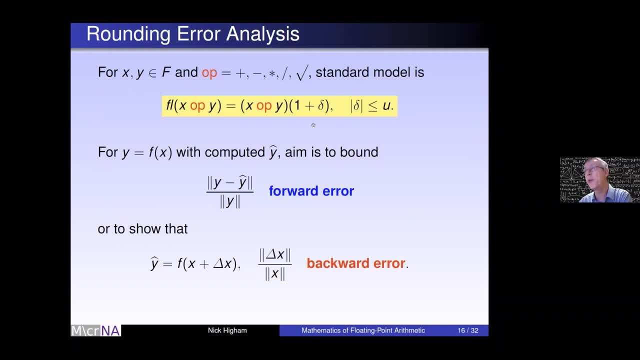 So again we just have a relative error of order u, whether we add, subtract, divide, multiply and similarly for the square root. And so what our overall aim is? in some calculation y is f of x. it's to bound either the forward error. so y hat denotes the computed solution. 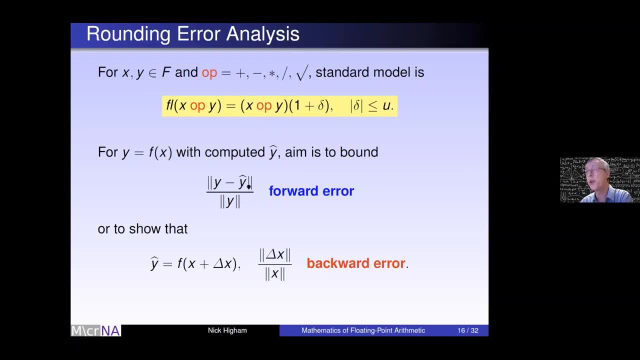 in floating point, and this could be a vector in general, or even a matrix. So this is the forward error, Or we want to look at the backward error, a notion that may be new to some of you, But this idea is that, rather than say what's the error, 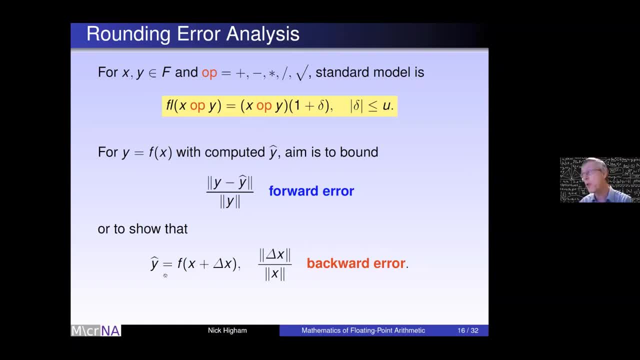 in y, we say: what problem have we actually solved? So how much do I have to perturb the data x in order that my computed y is the true solution, the true function of that perturbed data, And that's called the backward error? 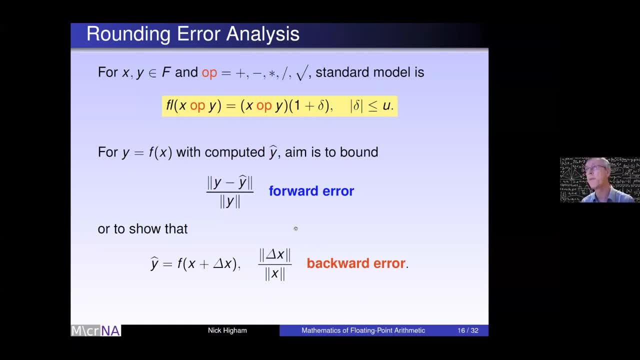 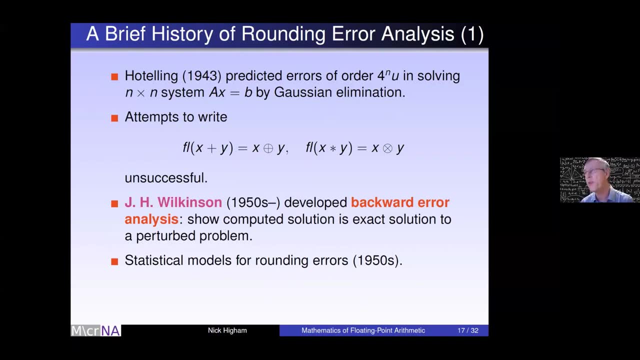 And this is just some suitable matrix or vector norm. Well, just a quick history of rounding analysis. Back in 1943, just before the first digital computers, Harold Hotling, a statistician in the US, predicted that if you solve an n by n system of equations by Gaussian elimination, 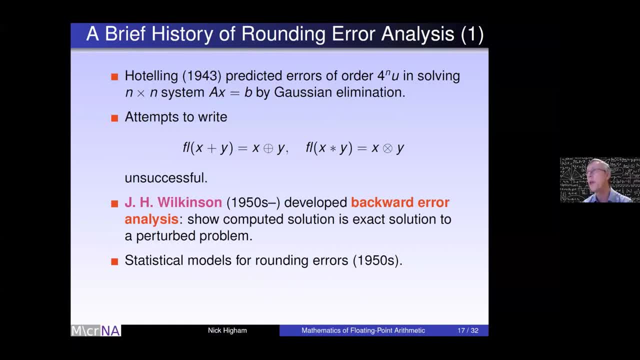 in floating point arithmetic that you would get errors of order 4 to the n times u, And this was quite worrying because, say, for double precision, this would mean n was limited to about 27.. So an extremely pessimistic viewpoint that worried a lot of people at the time. 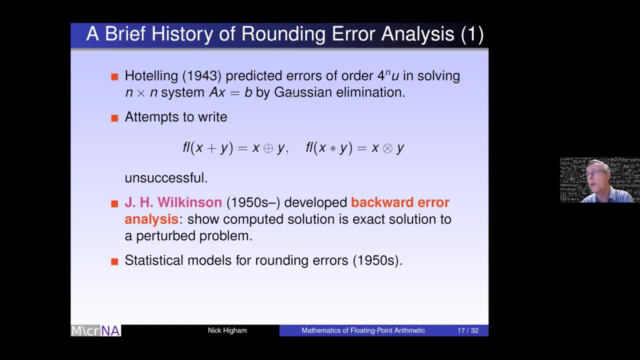 Early attempts to do rounding analysis and to understand the behavior of Gaussian elimination. some of them tried this approach. So let's think of the floating point addition of x and y as some new operator plus, which I'll put in a circle. So this means the floating point addition. 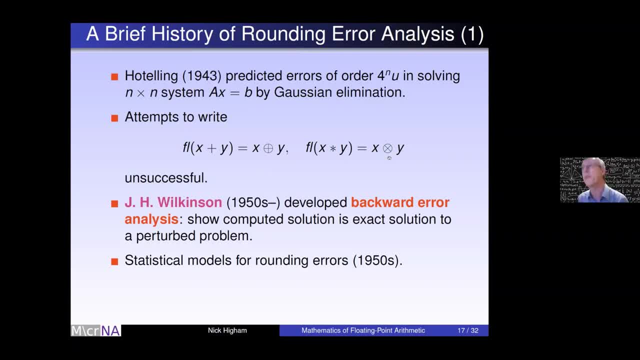 And similarly, times in a circle means the floating point times. So these are the results you get from your computer of doing addition and multiplication. So the idea is you take your algorithm, you replace every plus by a plus in a circle, every times by a times in a circle. 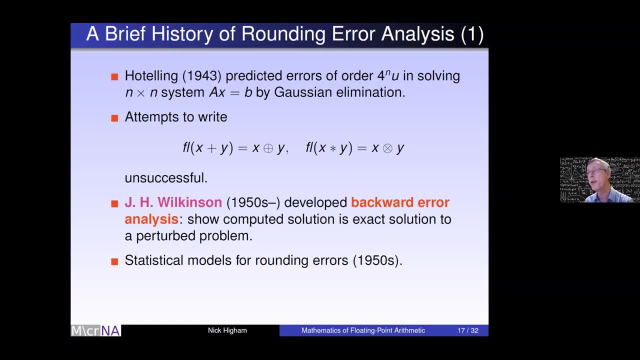 and so on, for divide and square root and subtract, And then just try and do the algebra to try and understand what is the accuracy of the final result. This doesn't work very well for a couple of reasons. The main reason is that, of course, 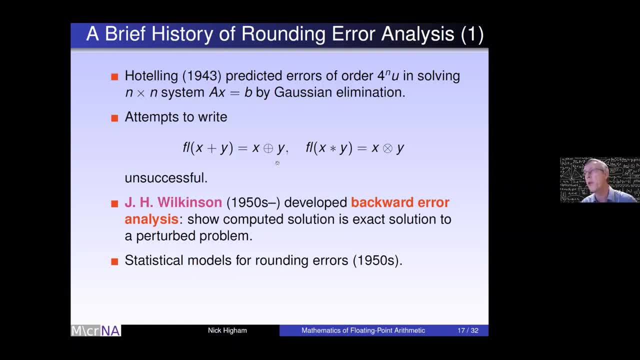 with this new algebra we don't have such nice relations. We know we no longer have associativity. Reciprocation is a bit dodgy, So all the things we used to doing no longer necessarily apply, And so it becomes very difficult to to do a correct calculation with these symbols. 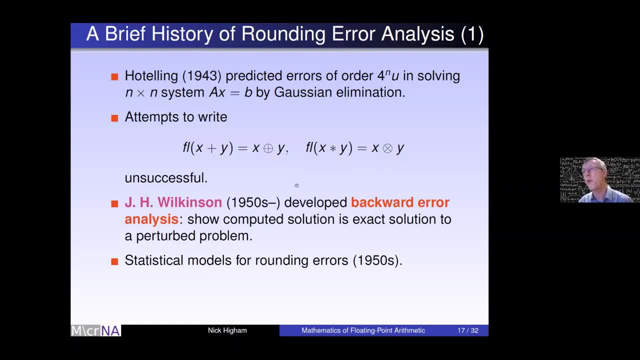 And the second reason it doesn't always work is that this inevitably leads you to a forwarder viewpoint And, as Jim Wilkinson showed in the 50s and 60s, backward error analysis is often the much more powerful way to go. So Wilkinson, based at the National Physical Lab in Teddington. 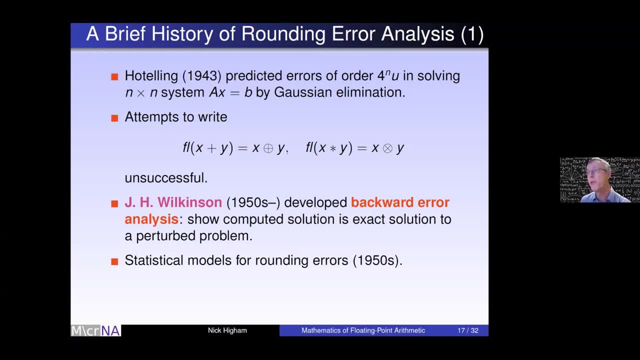 who is involved in building and developing the pilot ACE. after Turing left NPL. by using the pilot ACE from the 1950s onwards and doing the mathematical analysis of algorithms, he developed this idea of backward error analysis that I mentioned a moment ago. 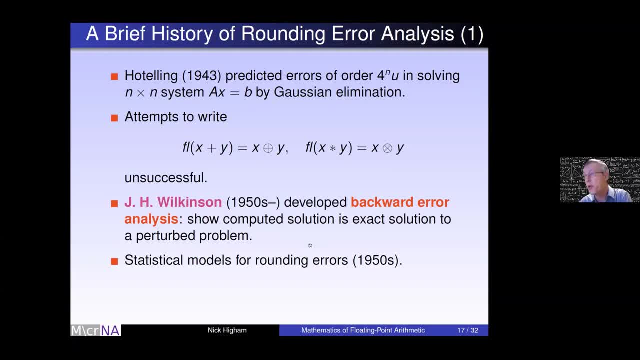 where you aim to show that the computed solution is the true solution to some perturbed problem, And so another thing that happened in the 50s was some proposals of statistical models, and I will come back to that in a moment, because that's sort of what I'll. 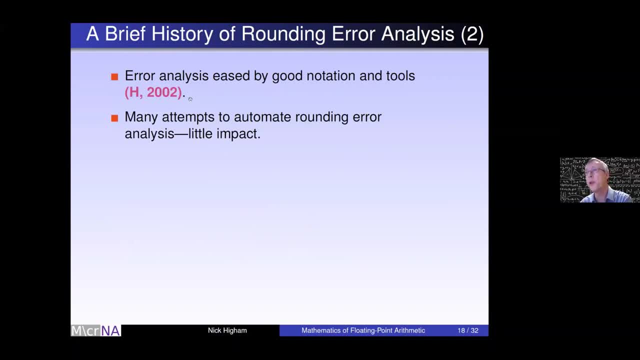 be talking about Jumping ahead to the present, my 2002 book, trying to synthesize all the different tools and notation and so on, And so what I present there is now pretty much how things are normally done, And I'll just say finally that in this history that there have been many attempts. 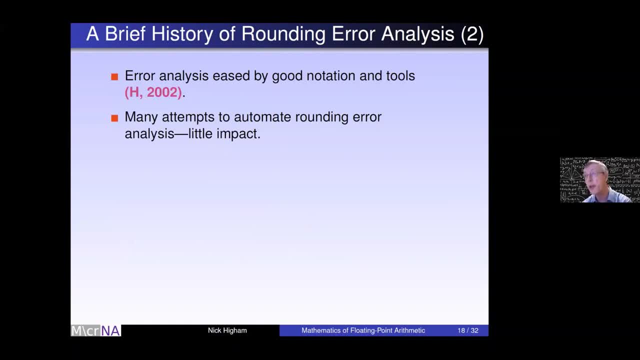 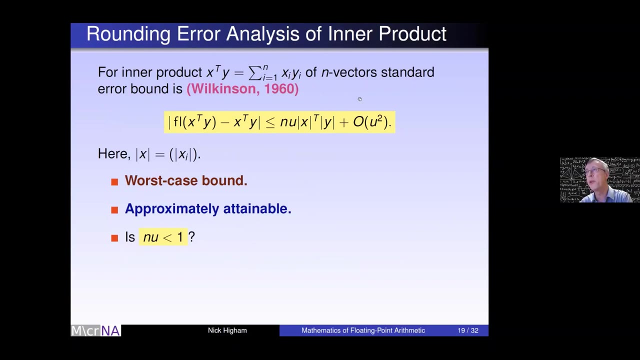 to automate everything, to make the computer do its own analysis of its own behavior, And that's really not been very successful. It seems to be very difficult to automate these things. You really need some human input and ingenuity. So let's just take a simple example of what Wilkinson was able to show for just 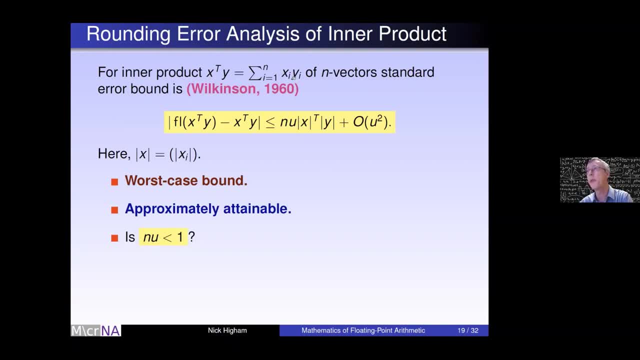 an inner product of two vectors. x and y are n vectors. We're forming this inner product. Wilkinson showed in 1960 that the error in the computed inner product is bounded in this way here When I write mod of the vector, I mean you take the modulus of the. 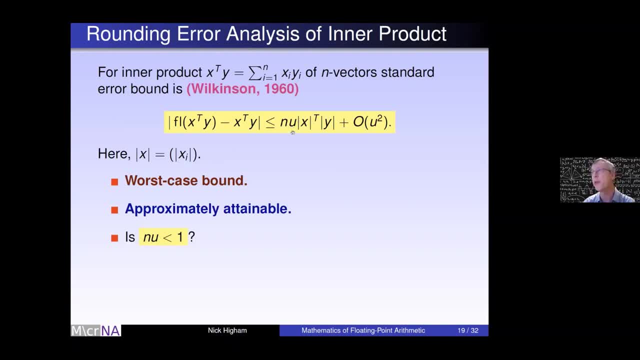 elements of the vector. Remember, use the unit round off. Think of that as 10 to the minus 16 for the moment. So the error is proportional to the number of terms times, the round off times, essentially the inner product. So this is a worst case bound. 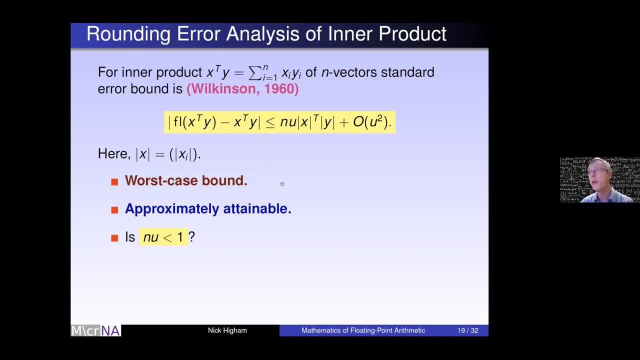 It's guaranteed that the error will not be bigger than that quantity. It is approximately attainable in the sense that you can find x, y and a set of rounding errors that will give you approximate equality here. So the question then is: or the first question, 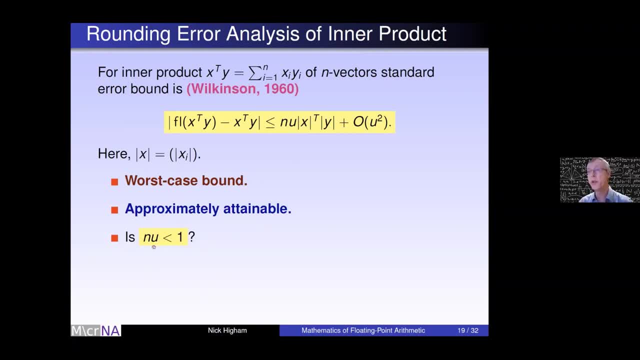 you might ask, is this bound telling us anything at all? Because we certainly need n? u less than one. Otherwise we're not guaranteeing even a relative error of order one. So we definitely need at least n? u less than one Now. in the past that wouldn't have been a big concern. 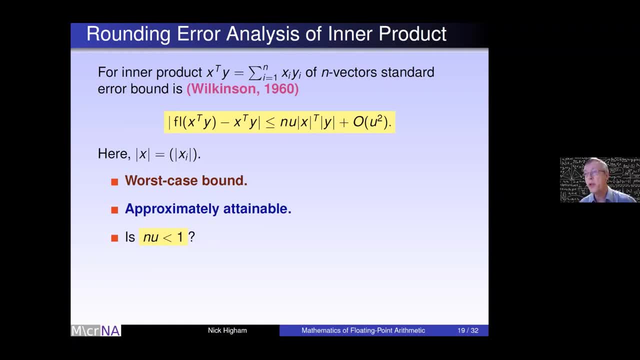 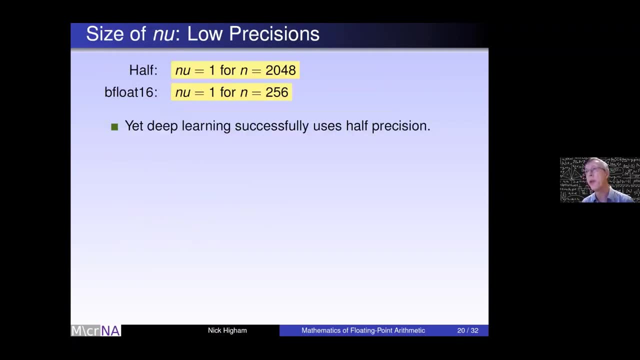 Now use 10 to the minus 16.. n is usually nowhere near 10 to the 16,, for example, if you're solving n equations and n unknowns, So normally you wouldn't bat an eyelid here. But nowadays we're looking at these low precisions. 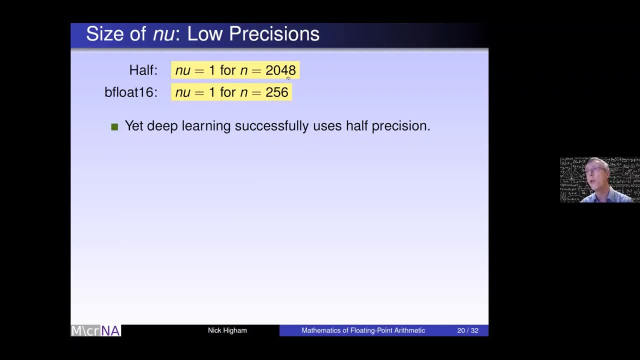 And unfortunately n? u is already one for n, a couple of thousand with the IEEE half, even 256 for the Google B? float And deep learning is using these precisions And it's definitely working within the products with more than this number of elements. So that raises the question of what is. 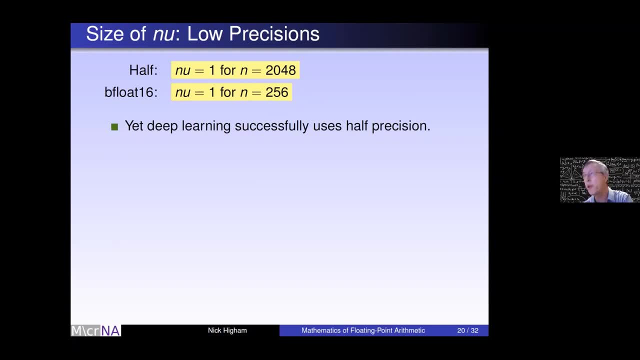 machine learning actually computing? Is it computing right answers? What's it actually getting mathematically? Well, Pete Stewart, a very distinguished numerical analyst, made a very nice statement And, rather like he said, to be realistic, we must prune away the unlikely. 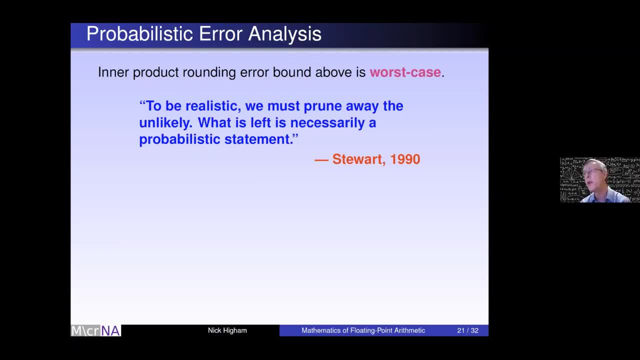 And so Wilkinson's bound that I quoted as a worst case bound. So Stewart says what we need is necessarily a probabilistic statement if we're going to get something that's more likely, more realistic, And in fact Wilkinson himself had already thought about this in the 60s. 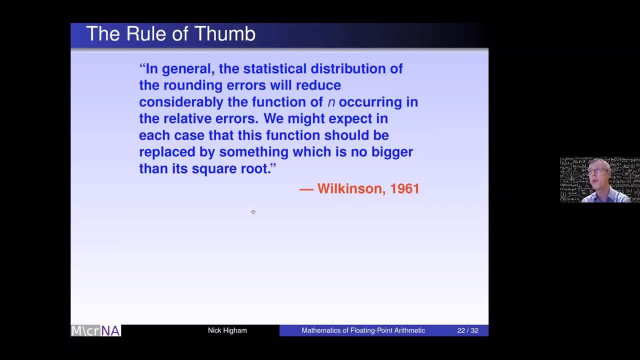 So he said here that the statistical distribution of rounding errors will tend to reduce considerably the function of n occurring in the relative. There are bounds, And we might expect that we could replace these constants by their square root, essentially. So, wherever you see an n root, n would be a more realistic. constant is what Wilkinson was saying. He didn't ever write this down formally, but it's clear what the thinking was. The thinking was based on the central limit theorem. We have lots of these tiny individual rounding errors, If we can assume they're independent, random variables and mean zero, and if any is. 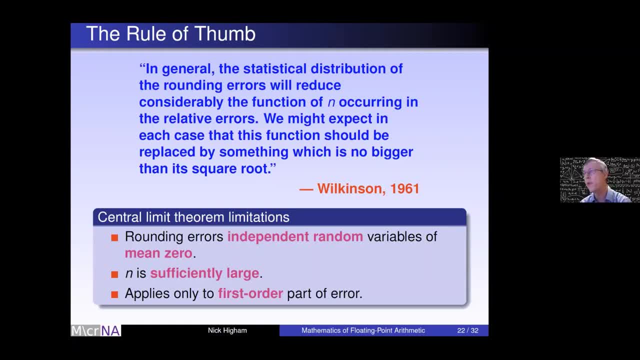 sufficiently large, then we can come to Wilkinson's conclusion here, at least for the first order part of the error, just by applying the central limit theorem. And the problems with this are that nobody's ever written this down rigorously. But perhaps the main, well, the two problems are, are these assumptions? 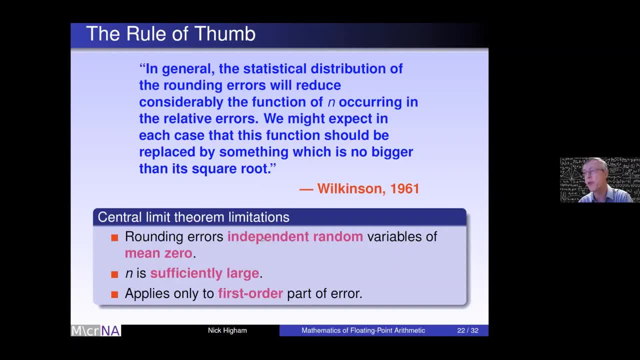 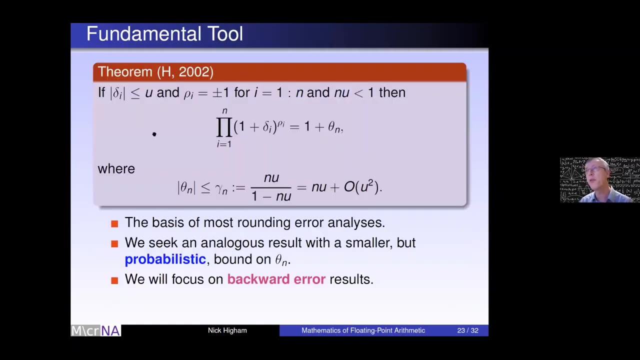 independent- here about the rounding errors being independent, random variables and mean zero. And what is a sufficiently large n? The central limit theorem doesn't tell you how large n has to be for this solution to be to be valid, So let me try and take a different approach. 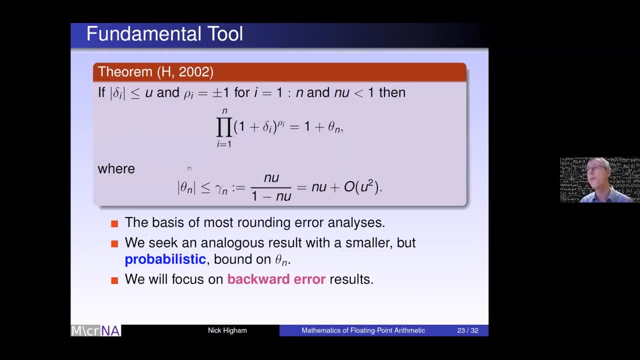 So what I'm showing you here is the just the usual or the standard lemma that this in my book that I tend to use when I'm doing any sort of error analysis, and it's just telling us what happens when you multiply lots of one plus delta terms. 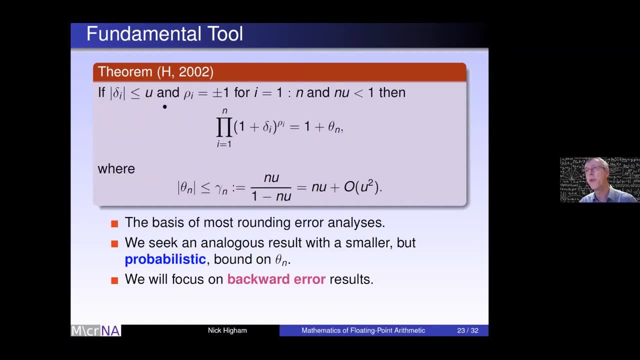 Each of these deltas is a rounding error. They're all bounded by the round off And it's giving us, it's telling us, how far away from one this product can be, And the main point is it's just a rather neat form of bound: NU over one minus NU. 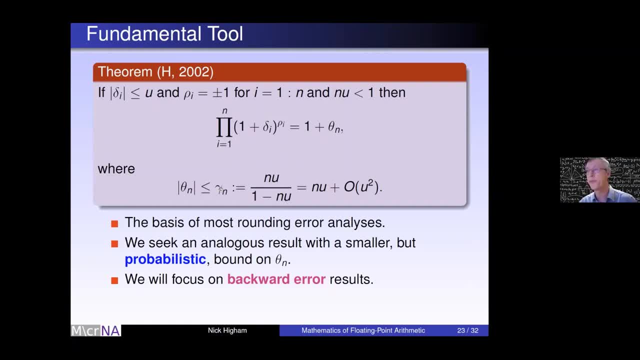 which captures both the first and higher order terms. So these gamma constants satisfy nice little algebra, which makes them easy to work with. So this is. you could say this is the basis of most rounding error analysis, This or something like it, because you will. 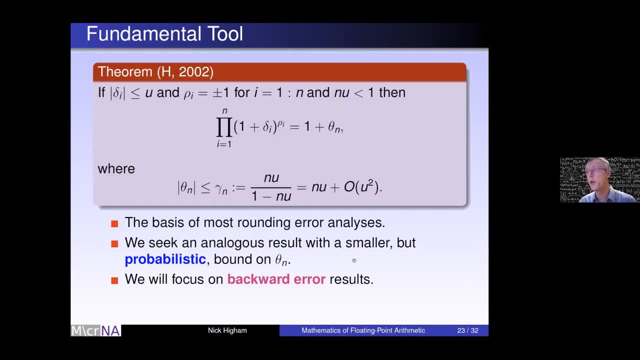 often get these products appearing in an analysis, So what I would like to do is to get a more realistic bound- This is a worst case bound. I'd like to get a probabilistic bound That I hope will be smaller, but I know I'll have to make some assumptions in order to get that. 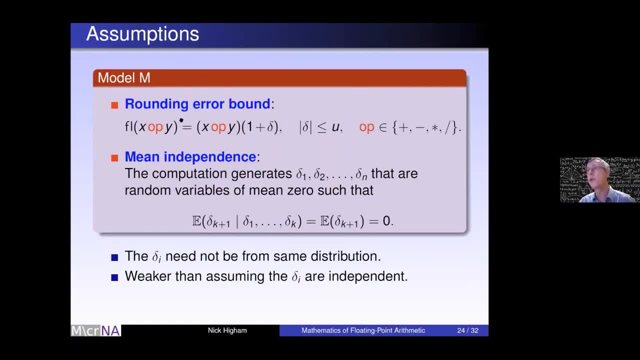 So here's a model I'm going to make use of. So I've got my rounding error bound as before, so that the individual rounding errors are still bounded by the unit round off. But I'm going to assume something else: that the computation generates rounding errors that are random variables. 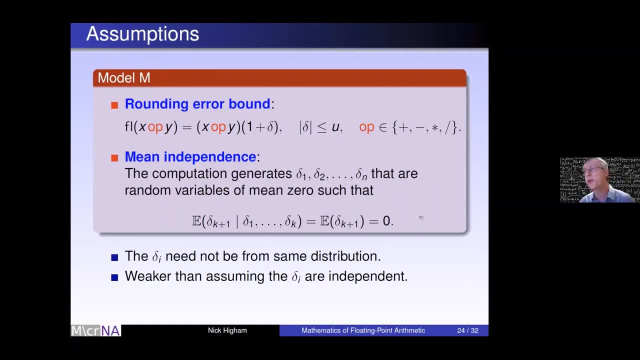 They do have mean zero. And then there's this mean independent assumption here. So it says that the k-plus first rounding error has expectation that doesn't depend on the previous rounding errors. That's this condition here. So that's mean independence, And certainly independence implies mean independence. 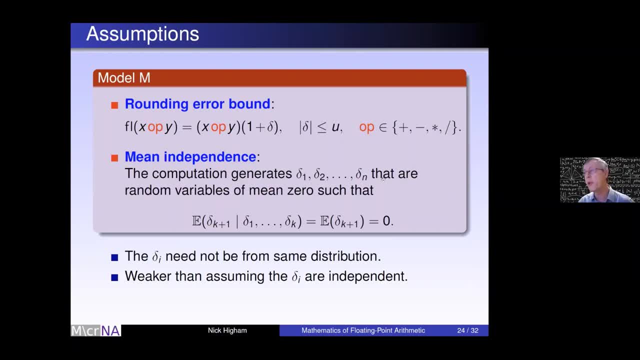 So this is weaker than assuming that the rounding errors are independent And the deltas don't even have to be from the same distribution for this model. So that's the model I'm going to take, and I want to see what I can do with it. 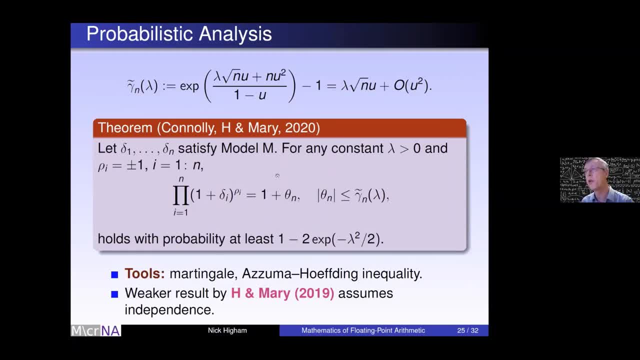 So this is a probabilistic version of the result I had two slides ago. It looks very similar, But now I'm assuming that the rounding errors satisfy the model. I have the same form of bound, but the upper bound on the theta here is a rather more complicated quantity. 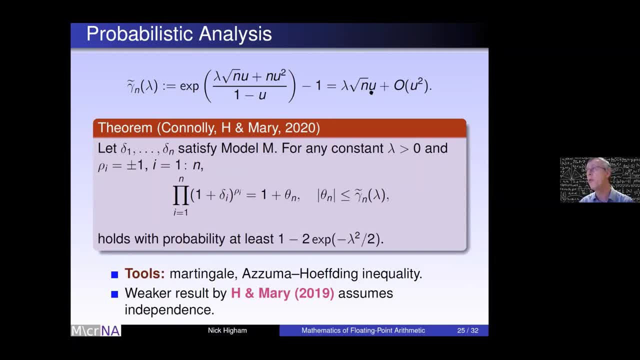 But the key thing is that, to first order, it's lambda root n. u Lambda, I'll explain in a moment. but that was n before, So the n has now become a root n, at the cost of this being a probabilistic bound. 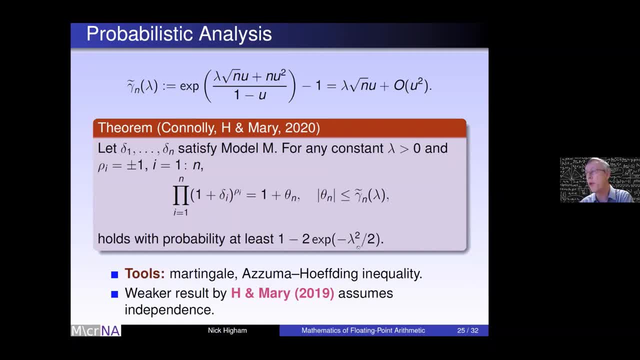 So we have a certain probability, at least this, of the bound holding And clearly the larger lambda is, the more likely the bound is to hold. but the larger lambda is, the bigger the bound is. However, lambda turns out not to really be an issue here. 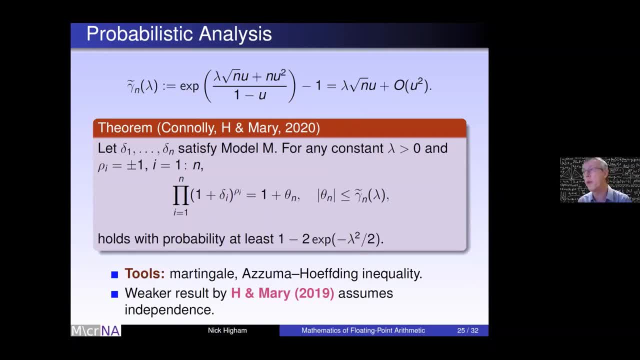 In practice, if we set lambda as 1, we find that the bound is always satisfied, So this is a probabilistic bound. The proof involves a martingale and this Azuma-Hurfting inequality, And Theo-Mary and myself had previously obtained a weaker result. 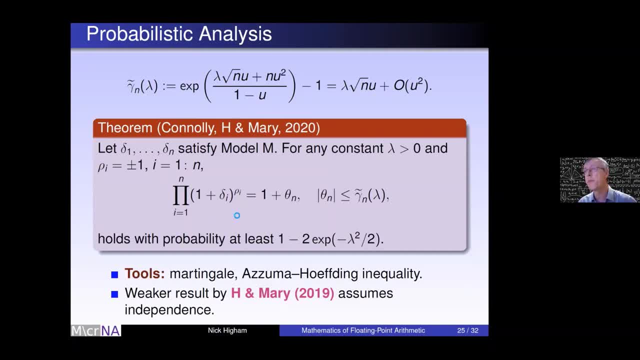 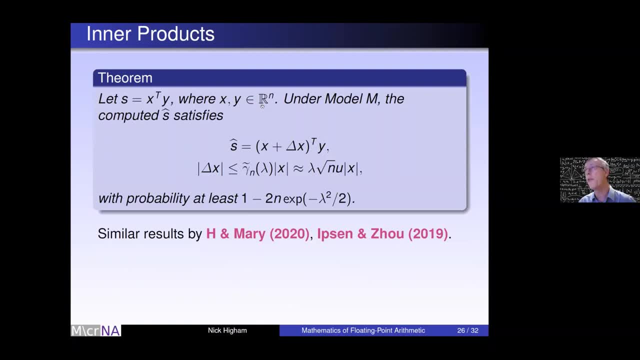 that assumed independence rather than mean independence. So if we apply that result to the inner product now, so same as before inner product to two n vectors Under this model, we now have this backward error bound. whereas before we had an n? u, here now we have lambda root n? u, with a certain probability. 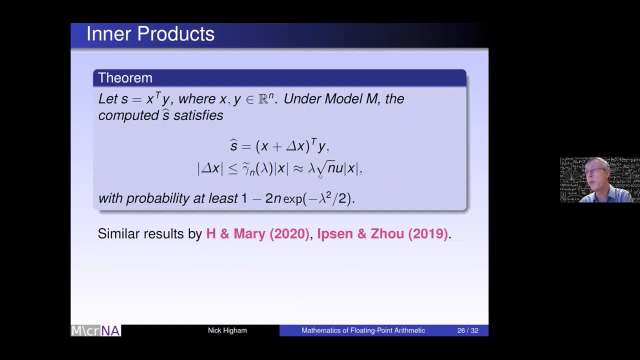 So the n has become a root n and the lambda isn't really going to be a problem. So this is now for large n. this is a much smaller bound, but it is probabilistic. That's for inner products. Once you understand inner products, you understand a lot. 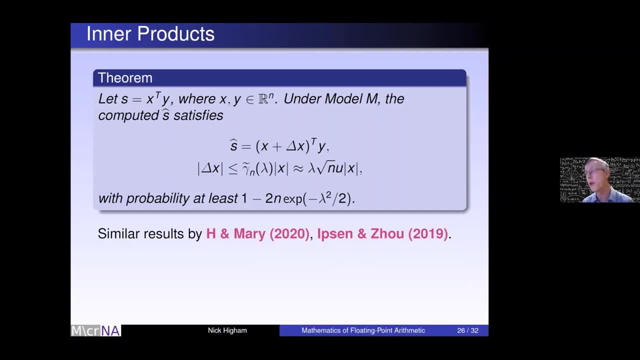 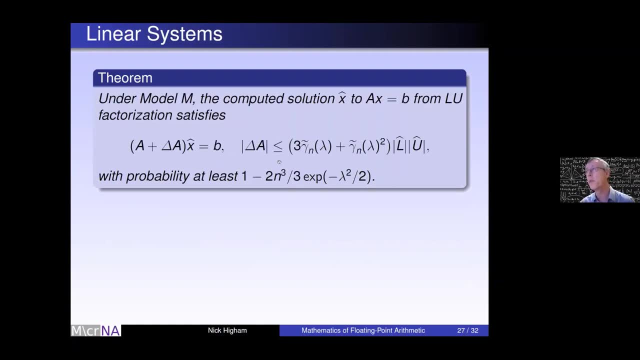 You can do matrix to products, you can do matrix matrix products and you can do Gaussian elimination, all really building on this result here. So I'll just show you the result for Gaussian elimination or LU factorization. That's the same thing. 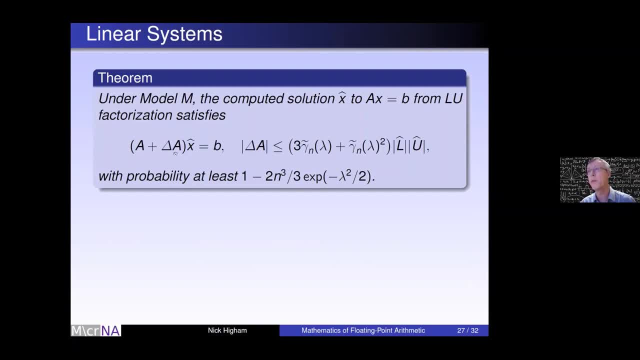 So you can show that the computed solution to the system solves a perturbed system, with this bound on the perturbation, And it involves the delta tilde which, remember, is proportional to root n times the unit round off. And we have this probability. 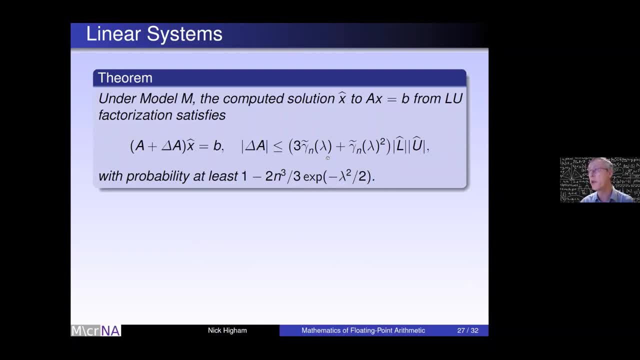 Again. so this is the same form as the classical bound, but whereas the classical bound would be roughly n? u, this is now roughly 3 root n? u. So just to be clear, what this has shown: this has really shown that Wilkinson's 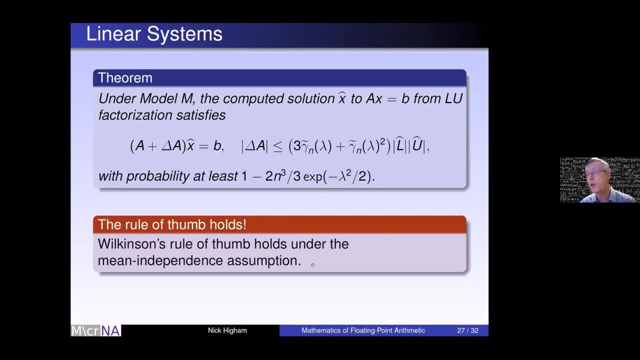 rule of thumb does hold under the mean independence assumption. So we've gone from an n factor here to a root n factor in gamma n tilde under our model, And this applies for any n, unlike the central limit theorem argument. Well, is this realistic? 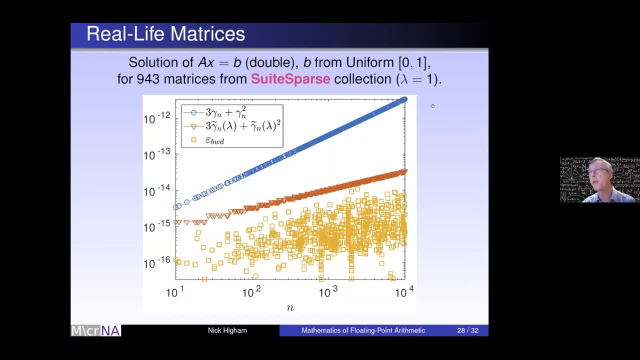 Let me just show you one set of results here. So these are some matrices from a collection called sweet sparse, maintained by Tim Davis, lots of real life matrices of all sorts of varying sizes. And what we've done is we've solved x equals b with a random right hand side. 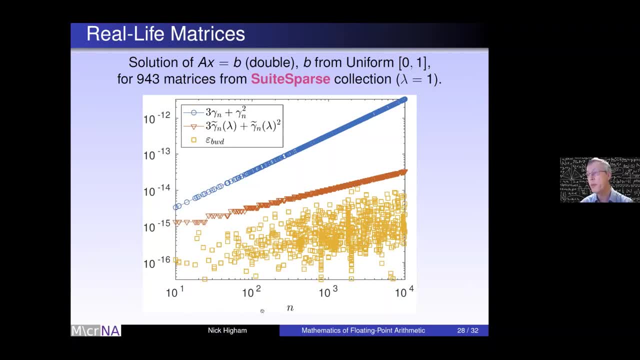 And we've computed the backward error which is shown in yellow. The dimension of the problem is on the x axis And the probabilistic bound from the previous slide is the red, the red triangles, And we can see that all the error errors are bounded by this bound and I've taken lambda is one to get the red line. 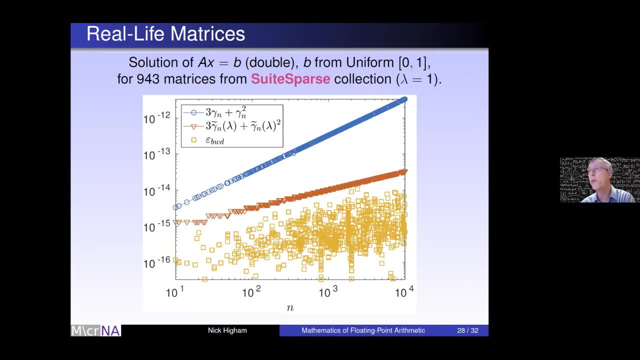 And so this: this is growing like root n? u and the blue line here is the traditional bound growing like n times u. So it's larger, it's faster growing And the probabilistic bound is clearly a much better predictor of the actual backward error. 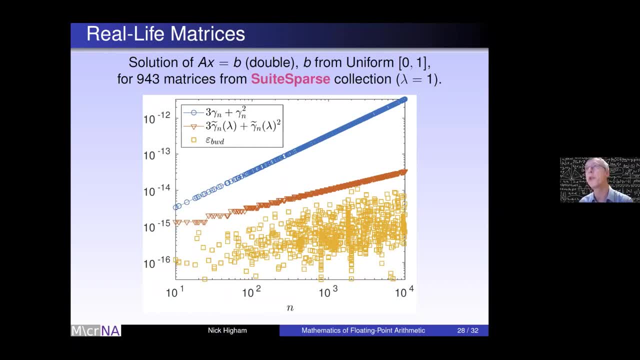 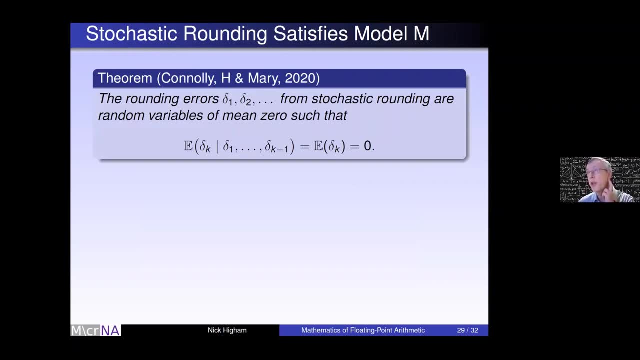 for this problem, computed with round to nearest in in double precision. Let me turn now back to stochastic rounding, because I mentioned this at the start. What's the role of stochastic rounding in all this? Well, it turns out that stochastic rounding automatically satisfies the model. 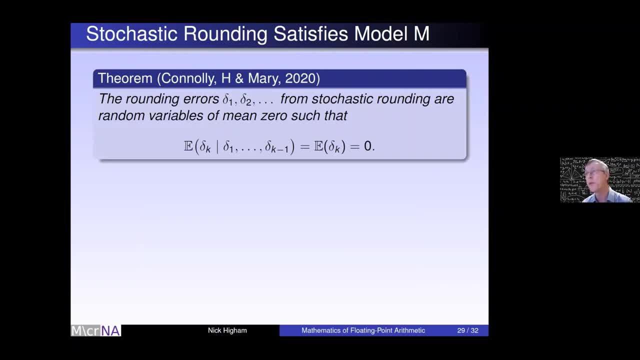 So, remember, it is by definition probabilistic, So the rounding errors are random variables And it turns out they have mean zero And they also satisfy this mean independence assumption. This just comes from the definition of stochastic rounding, So that means stochastic. 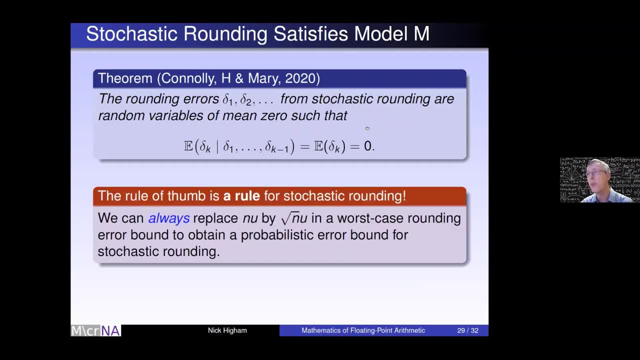 Rounding satisfies our model M, And so the rule of thumb- Wilkinson's rule of thumb- is always true for stochastic rounding. Now there's no further assumptions required. We can always replace n? u by root n? u in a worst case, bound. 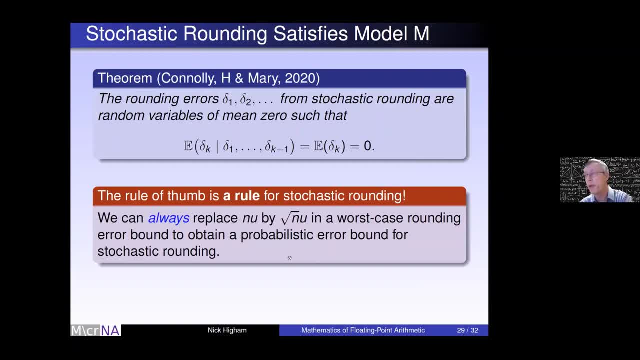 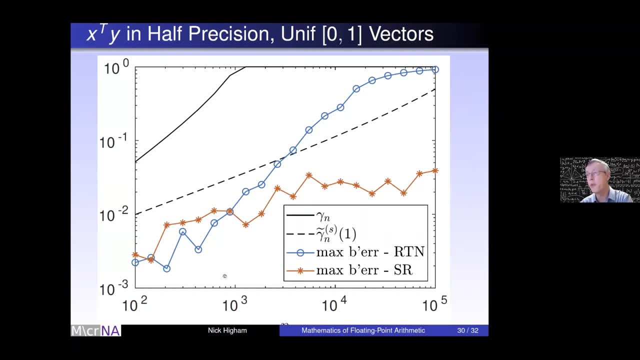 to get a probabilistic error bound, with some specified lower bound on the probability of the bound holding. So let me show an example to illustrate this. So here we have an inner product of two vectors with elements drawn randomly from the uniform distribution on 0, 1.. 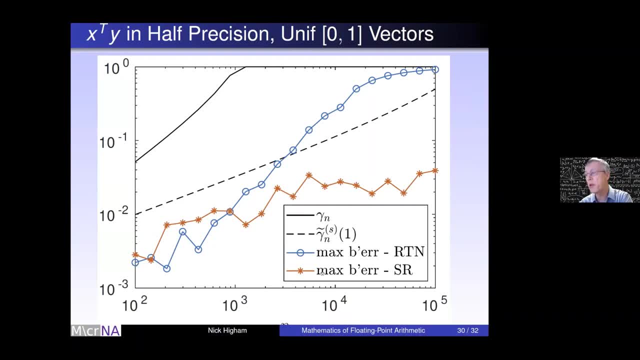 And what I'm plotting for n on the x-axis. I'm plotting the error for round to nearest. This is the blue circles, OK, and I've got the error for stochastic rounding the red or orange stars. So initially, round to nearest is a little bit more accurate. 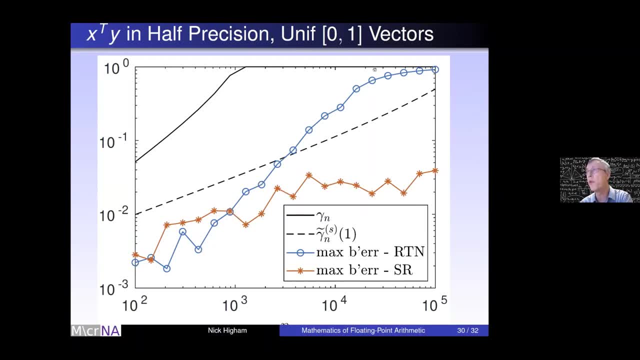 But after a while the error starts to grow. We cross over And before long we've got errors of order 1 for round to nearest, Whereas with stochastic rounding the errors are much more slowly growing and we still have a couple of digits of accuracy by the time we get to. n is 10. 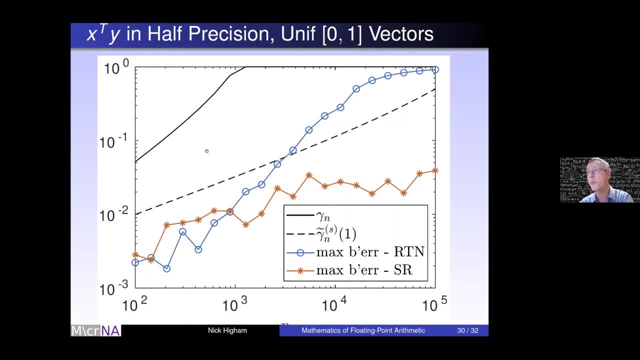 to the 5.. So this is in half precision. The solid black line is the traditional worst case bound and that quickly approaches 1 and does indeed bound the error with round to nearest. The dotted line is the bound for stochastic rounding Which grows like root NU. 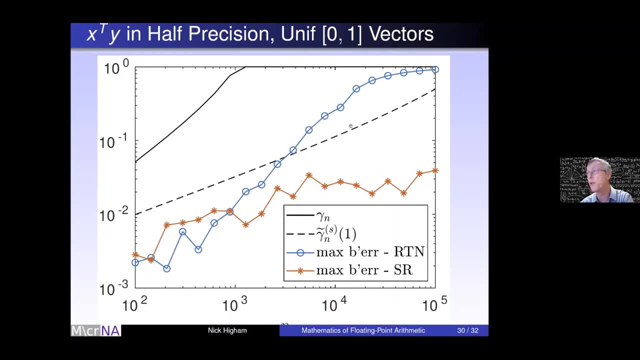 And you can see that round to nearest fairly quickly starts to violate this root NU bound. So the question is: why is round to nearest doing so badly and why does it violate the bound? If its rounding errors satisfy the model, then it ought to be below this dotted line. 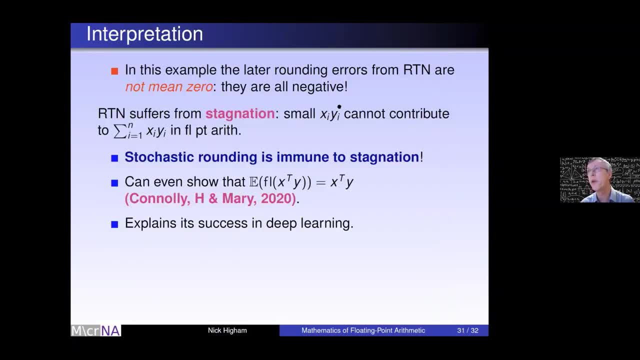 But clearly it's not satisfying the model. So what's going on? Well, it turns out that the rounding errors in the later stages of this computation are certainly not mean zero, as they would need to be for the model. In fact, they're all negative for round to nearest. 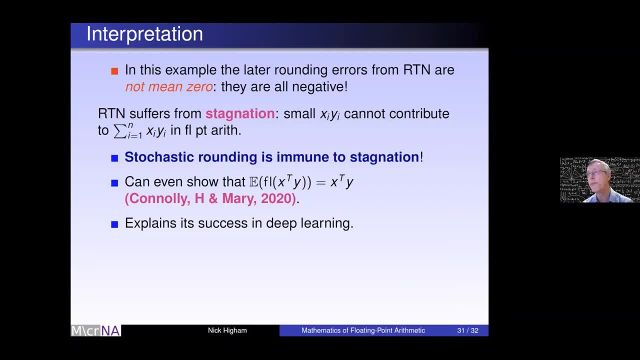 The reason is we're adding a sum of non-negative terms And so the partial sums are gradually growing, whereas the terms we're adding are all bounded by 1. So eventually the terms we're adding cannot change that partial sum because we have a large number of terms. So you add a new term with round to nearest. 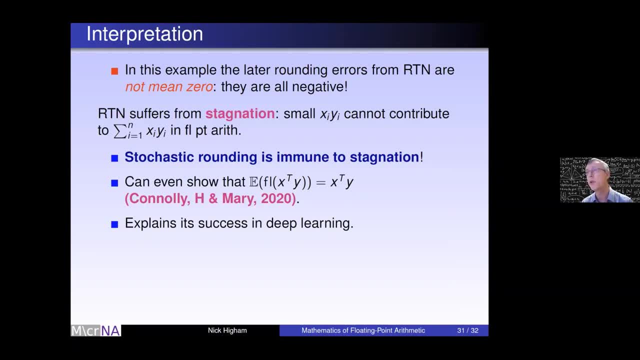 it just rounds down back to the original value. So it should have increased the value a little bit. It's not done. Therefore, the rounding error is negative. So from a certain point onwards, all the errors are negative and the model is violated. 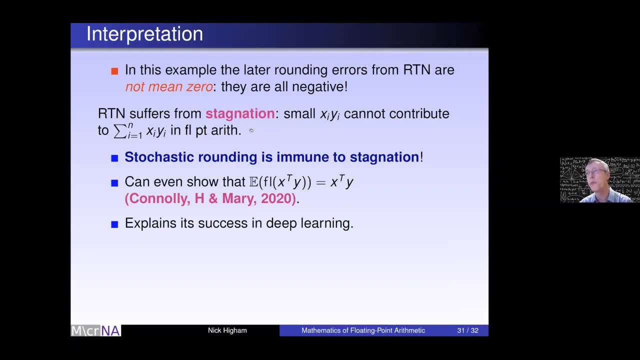 So this is what we call stagnation: when you have a sum of non-negative terms and when, eventually, with round to nearest, you're not increasing the sum any further. So that means that small products cannot contribute to the sum with round to nearest. Stochastic rounding, though, doesn't suffer from this. And the reason is really by its definition: every now and then stochastic rounding will round up. even if that's low probability, It's just enough probability of happening to give a rounding error of a different sign And that's just enough to give this. 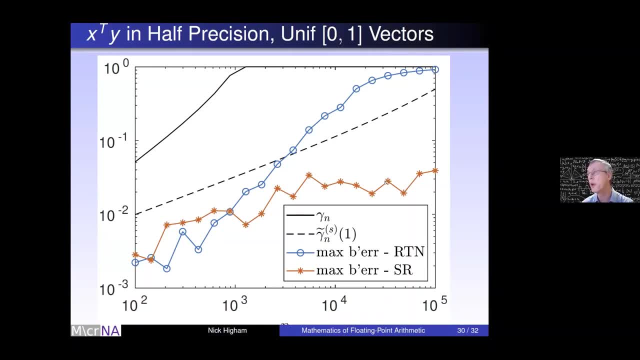 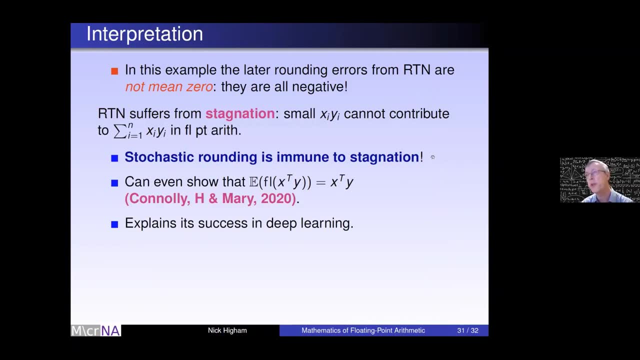 behavior we saw here where the errors are really quite slow growing. So that's really a nice feature. So by giving up the sort of greedy aspect of the rounding, we're benefiting from the more global picture of rounding errors being allowed to cancel and allowing to give us a much more accurate answer. 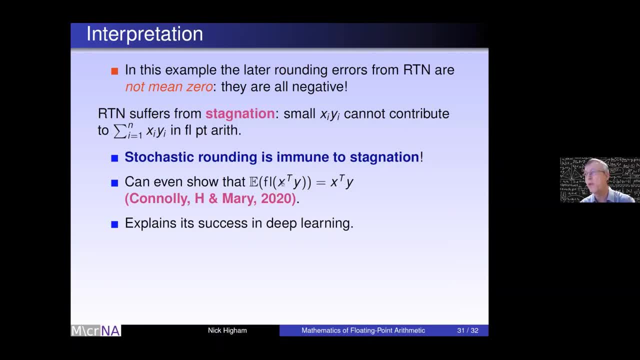 Another way of looking at it. this is to say, what is the expectation of the computed sum? So, mathematically, the expectation of the computed sum with stochastic rounding is actually the exact value. It is X transpose Y and we can prove that. 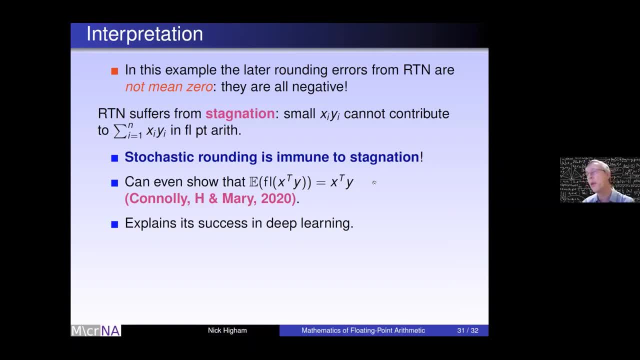 So this is another way of seeing why stochastic rounding, with its ability to go either way with these varying probabilities, that can benefit you in the long run on a long computation. And so I've written down here this explains the success in deep learning. So what I mean by that is that in deep learning, when you're doing 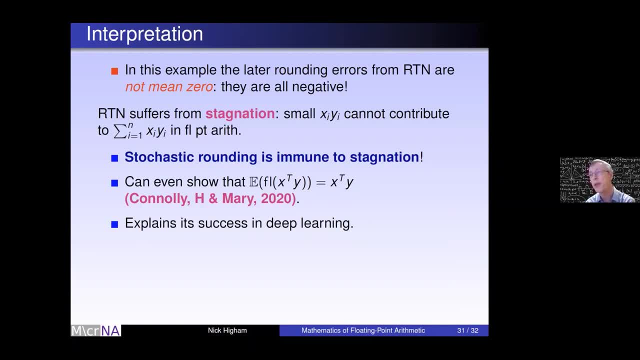 the stochastic gradient algorithm. you have parameters that you're gradually updating with a steepest descent, like method, And I think what happens in practice is the step size you decrease. you're adding smaller and smaller increments to an existing quantity And this is why 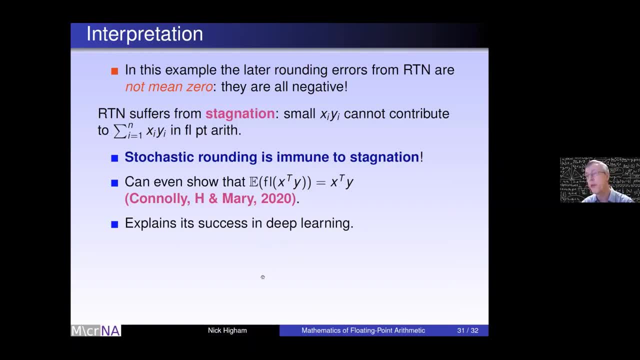 machine learning researchers are liking stochastic rounding because it does allow those, those later updates, to actually change the value and avoid what would otherwise be a stagnation. And they are working typically on these low precisions which run very, very fast in hardware. And it's a low precision where you really see this affect the most of stagnation. 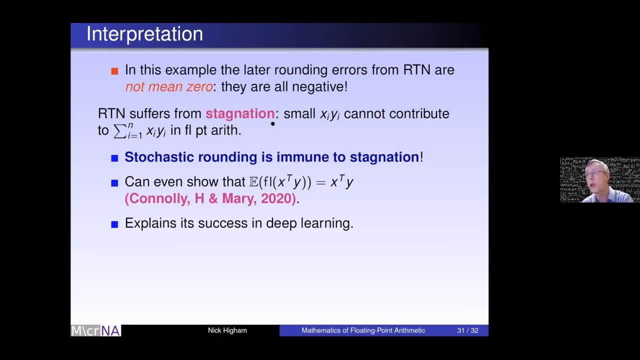 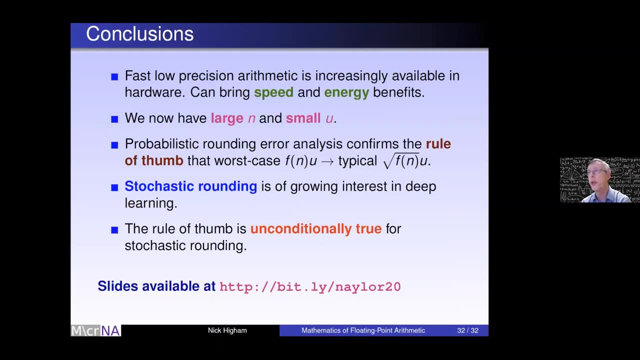 because n doesn't have to be all that large for stagnation to actually happen. So conclusions then? So we're seeing more and more in hardware now low precision being supported, certainly in GPUs, graphical processing units, Intel's next generation of desktop chips. 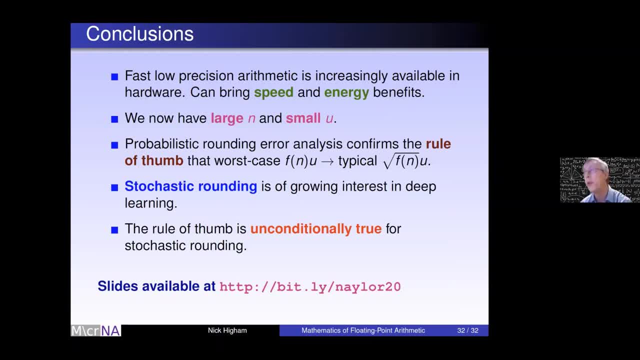 I think we'll have IEEE half precision or BFloat 16 in them, So before long we will all have access to this fast, low precision through our favorite software package. And the reason it's so exciting to people who do a lot of computation is not. 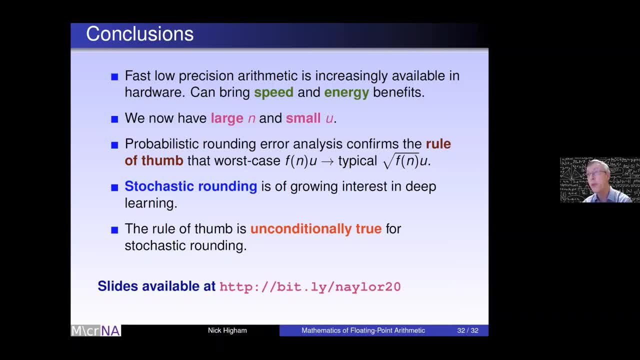 only is low precision, faster, it involves less memory movement, which is also a benefit to computation, and has lower energy requirements. So it really wins on all sides, except, of course, accuracy. So the one thing you're giving up is the accuracy of the results. 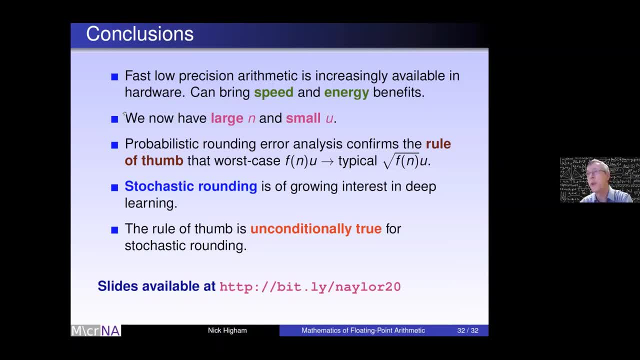 And so we have to be very careful to make sure that we are, that our overall computations are still reliable. So another way of saying it: we've got. we've got large n. n is always growing in practical problems, but u unfortunately now is getting smaller. 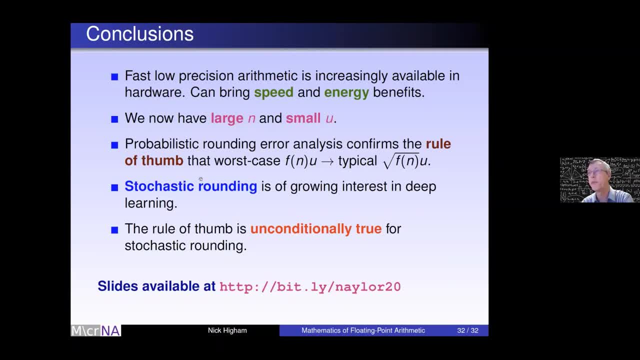 And so the product is something we really have to worry about. The probabilistic analysis I showed you confirms that rule of thumb- The first put forth by Wilkinson in the 60s- which says that, on a sort of statistical argument, the worst case bound can be. 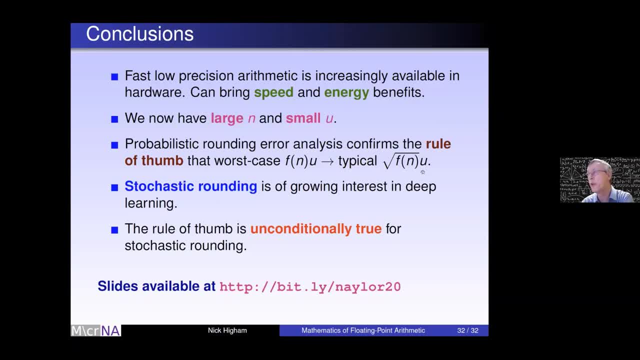 expected to be more like the root of the constant in practice. So an n would become a root n, And that's certainly a big benefit. But for round to nearest this isn't always valid, as we saw in the last numerical example. 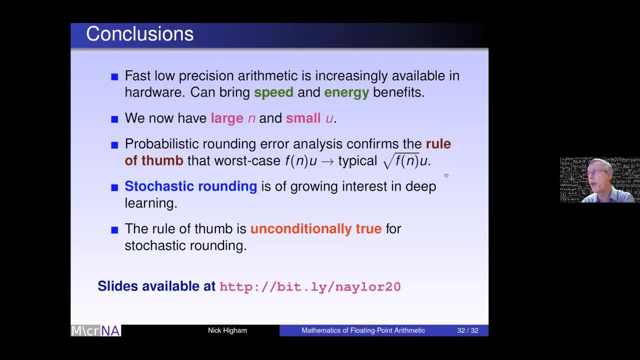 So the beauty of stochastic rounding is it always has this root n effect. There's no further assumptions needed. The probabilistic nature of stochastic rounding automatically gives you this reduction in the constant and automatically gives you the ability to avoid stagnation and have the correct expected value for the computation. 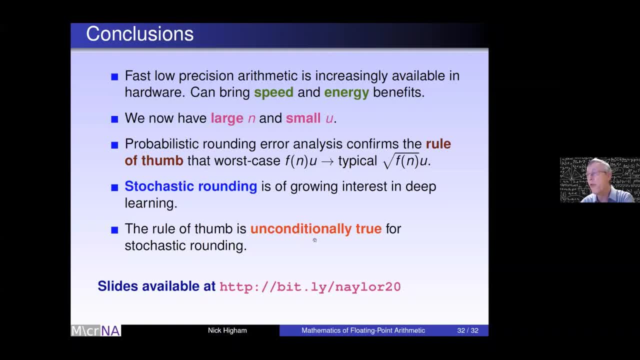 So another way of saying it is the rule of thumb. Wilkinson's rule of thumb is unconditionally true with stochastic rounding, So I think it'll be interesting to see how stochastic rounding plays out in the future. as we get more and more hardware implementing low precision, we'll need to think of more and more clever ways. 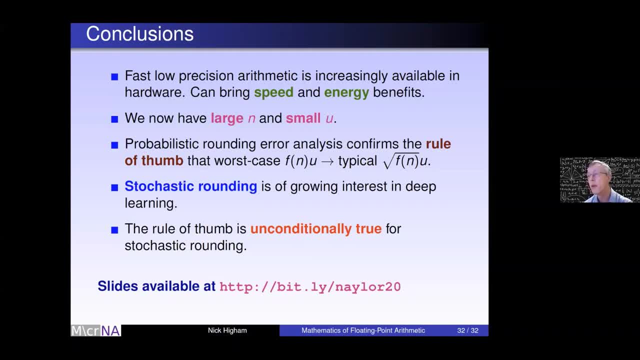 that we can exploit that hardware, And this different form of rounding is certainly one attractive way, I think, to do that. OK, I think I'll finish there. Thank you, Nick. thank you very much for a most beautiful lecture. It's wonderful to see how. 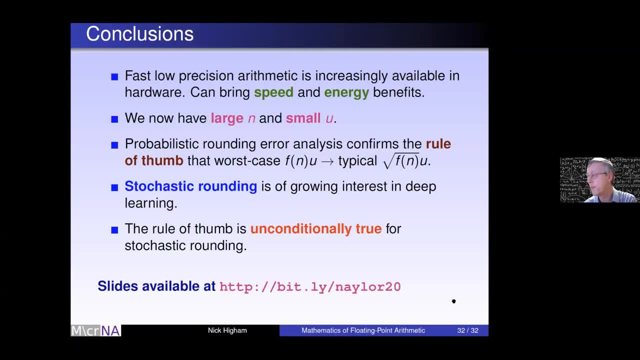 questions that are of enormous practical interest, of course, as we understand in many contexts, in all such beautiful mathematics And we have time for questions. So if you have a question for Nick about his lecture, please do type that now into the into the chat facility. 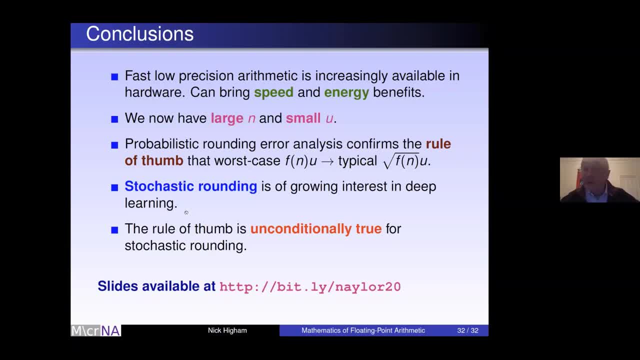 We have plenty of questions, in fact, So please do feel free to fire your questions in while people are typing or are developing their ideas on this. So you, this analysis involves some sort of central limit theorem, Nick, but what about the sort of large deviations? 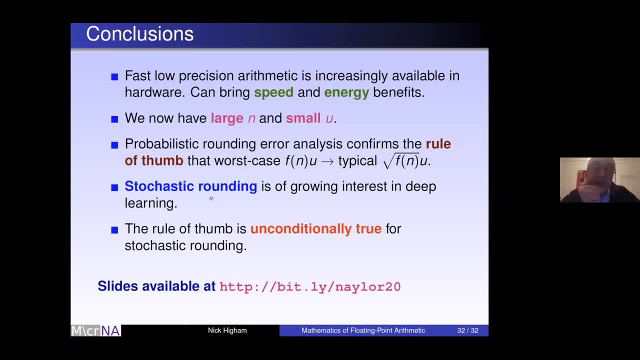 Is there some regime where you can ask about probabilities of attracting very large errors and how those might scale? Well, that's a good question. I should say I'm certainly not an expert on probability, so I've learned a lot in doing this work. 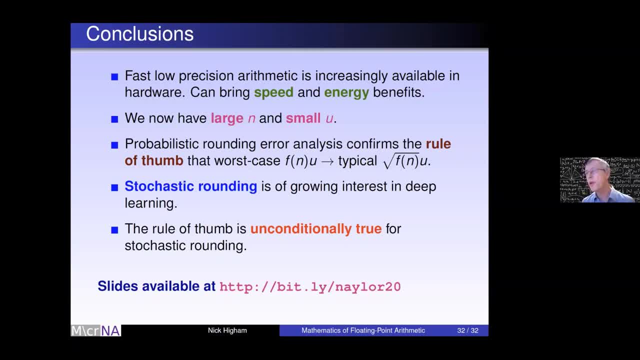 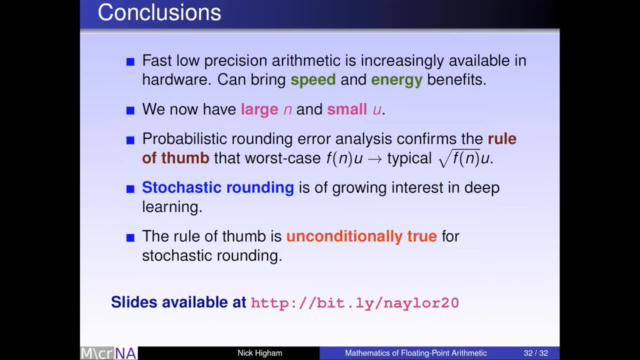 I didn't know about Concentration, inequalities, martingales and things like that. So we've taken one approach and I'm sure there's much more to be gained by combining some probabilistic theory with numerical arguments. So that sort of thing is probably wide open for people to have. 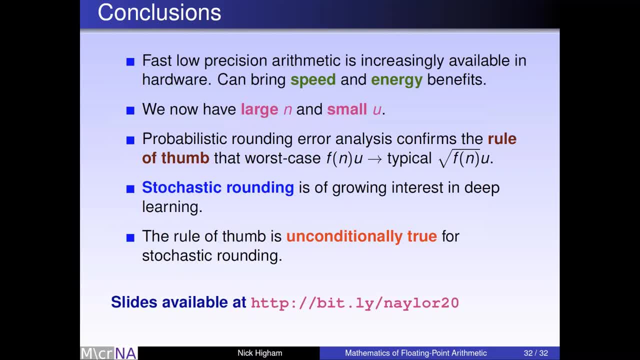 a look at and hopefully get some some useful results, I think, Good. So we have a number of questions coming in One: how good does pseudo random number need to be for stochastic rounding success to be successful? Oh yes, Thank you for asking about that. 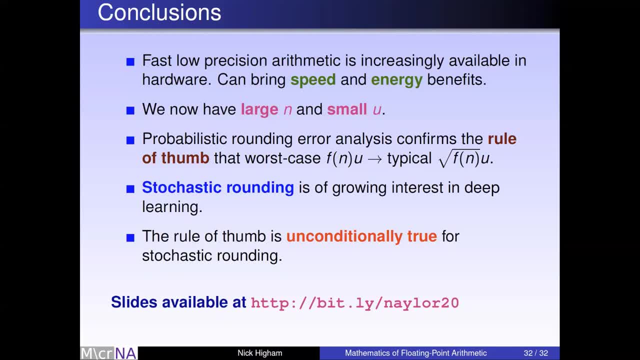 because the thing I haven't said anything about is how you actually implement stochastic rounding and actually it is not at all trivial If you think about it the way I've defined it. you need to know, You need to know those nearest floating point numbers and you need to have some way of forming that. 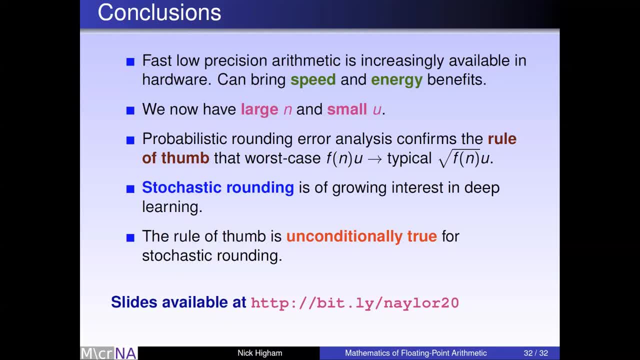 that probability. So implementation is not at all trivial. If you have a high precision arithmetic, you can use that in an obvious way to implement stochastic rounding. If you're already at the highest precision, then that's another question. So this is very much an open question. 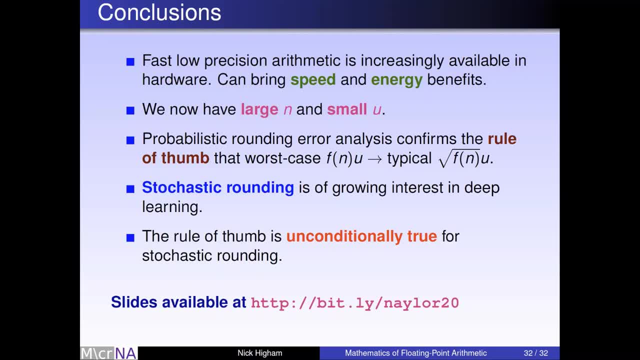 My colleagues in Manchester, including Mantas Mikaitis and Max Fassi, are looking at this. in fact, have some work on this at the moment. So how to efficiently implement stochastic rounding is not clear. How good the random number generator has to be also is something. 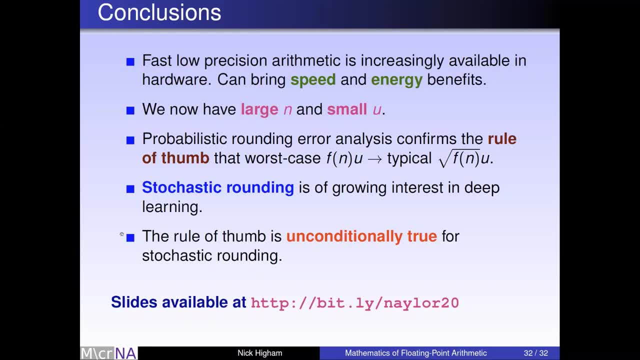 Michael Connolly has been looking at. So again, that's not trivial. You would hope that you can get away with a fairly low accuracy random number, but quantifying that is certainly needs some very, very careful analysis. Good, So we have another question from Martin Hira. 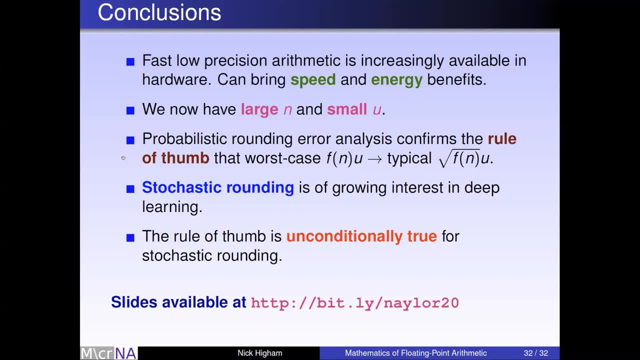 Generating random numbers is usually very expensive. How does stochastic rounding get around this? Yeah, so I can answer that in one sense In hardware, in some hardware, I think the 1950s paper I mentioned, because these people are designing the hardware they're able to essentially get. 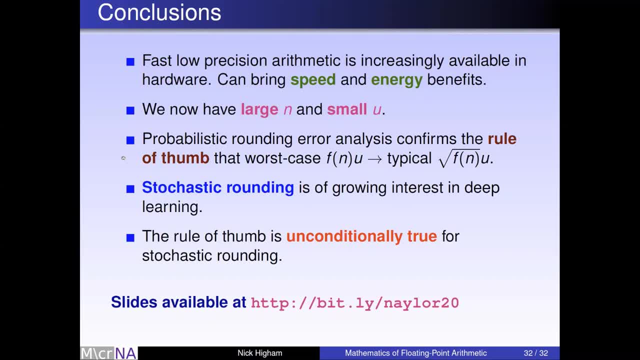 the randomness from the hardware, from the way that things are done in hardware, And the same is true of colleagues in Manchester working on the Spinnaker machine, where they're designing the chips that do the modeling of the spiking neurons, And so they're able to make use of what's. 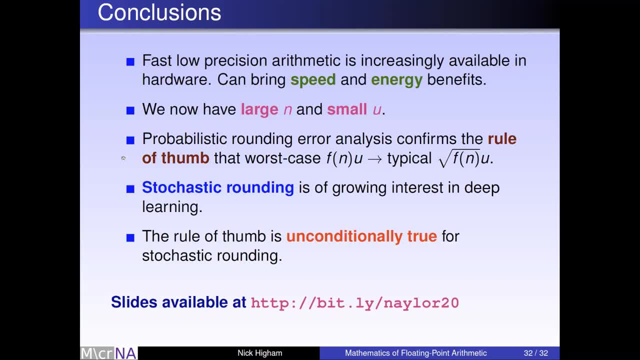 going on in the background to get some inkling of what these random numbers can be And to make the whole thing more efficient. But if we're working in a typical programming language where we don't have access to the underlying very, very low level details, this is clearly going to be harder. 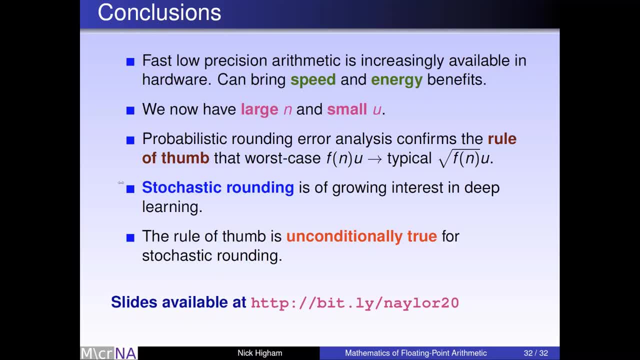 And yes, that's an open question: How much? what can you do efficiently? How accurate do your random numbers have to be? How much precision do they need? All these things are open questions. What's done in deep learning? I'm not sure. 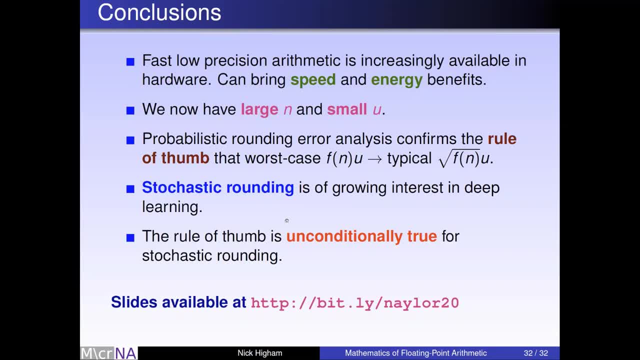 The problem with the deep learning papers I've looked at is that they very rarely give any much detail at all. So I think you would really have to go and look at the actual software they're running to try and find out what's going on in the background. 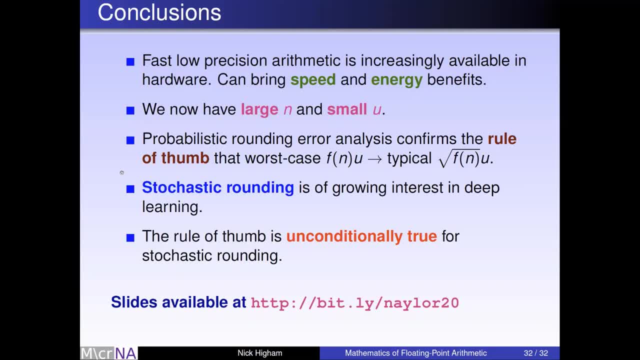 So I don't really know how it's done in the in the deep learning papers I referenced. Good, And a question from Aria Isilis: Is there a connection between this framework and one, smooth complexity analysis of Spielmann and two, concentration of measure? 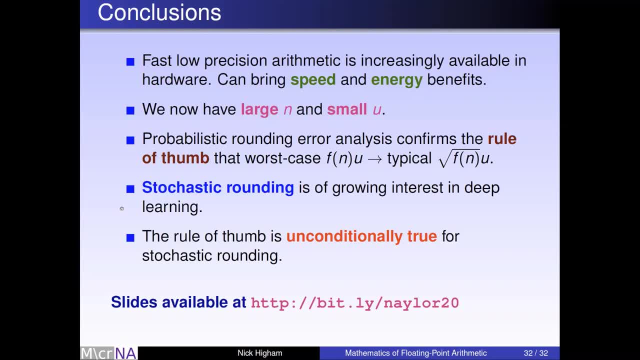 Not that I'm aware of The first one I know a tiny bit about. I'm not aware of the connection Concentration of measure. I'm not too familiar with that at all, So I really don't know if there's a connection with that one. 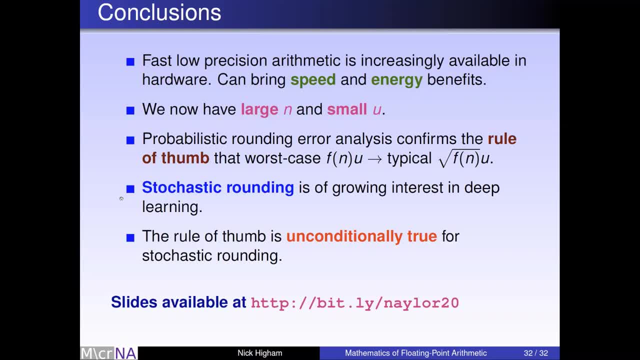 OK, so a question from Michael Overton: is it important that the probability of choosing to round up or down depends on how close the true answer is to the upper or lower band? what if you choose a 50-50 decision? Oh, thanks again. Yes, 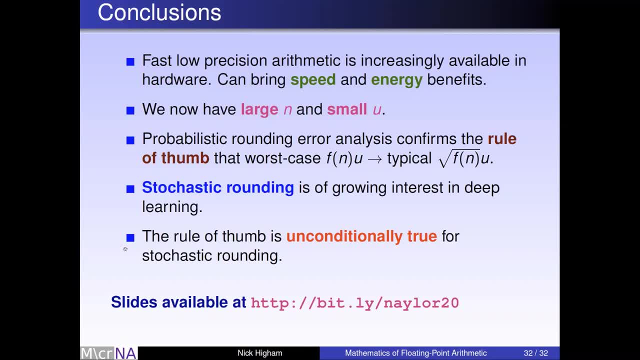 Again, I could have mentioned that, but I didn't. So there's another form of stochastic rounding, which is where, rather than do it with this proportionality, you simply say: I'll go up, you toss a coin, I'll go up if it comes heads. 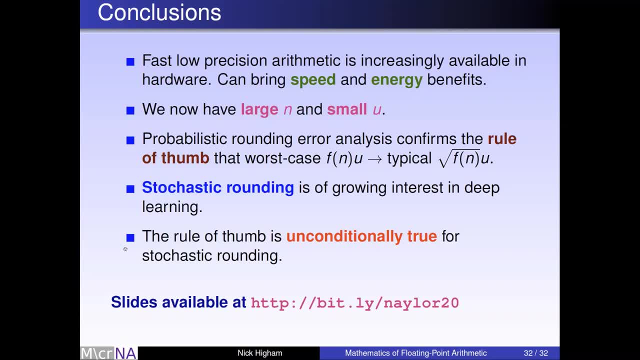 Otherwise I'll go down. So you have a 50-50 chance of going up or down, irrespective of how close you are to those two nearest floating point numbers, And so that is a method that is used in rather different contexts- The French school of Venia, for example. 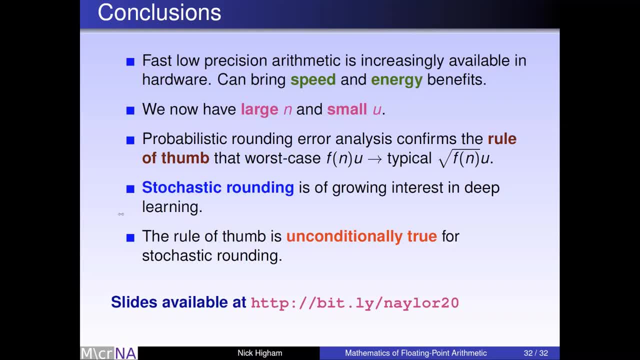 have used that over many years in their software packages that try to assess the reliability of the software. So that's a very different flavor to what I'm talking about here And that type of stochastic rounding doesn't really have the same probabilistic properties like zero mean, for example. 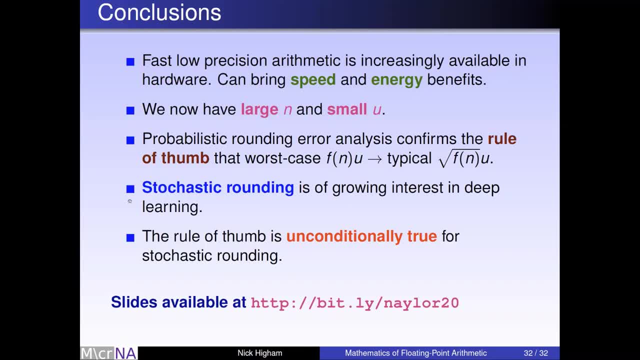 So, yes, you can do that, and people do do it in different contexts, But I think here it doesn't have these nice properties that I've been talking about, in particular this, you know, satisfying this Model M that I've referred to here.